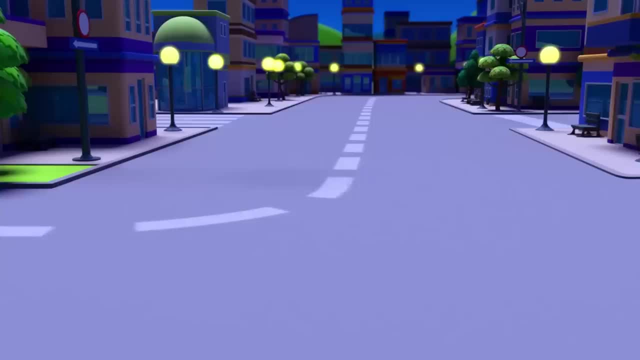 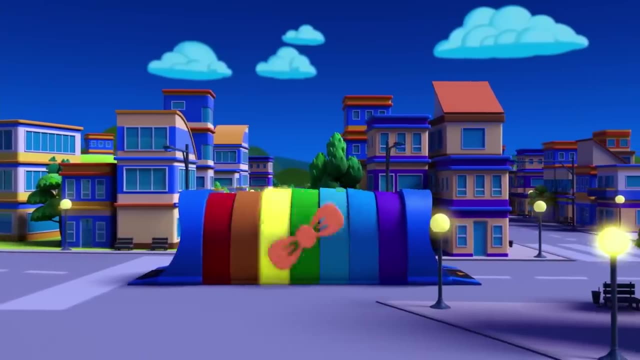 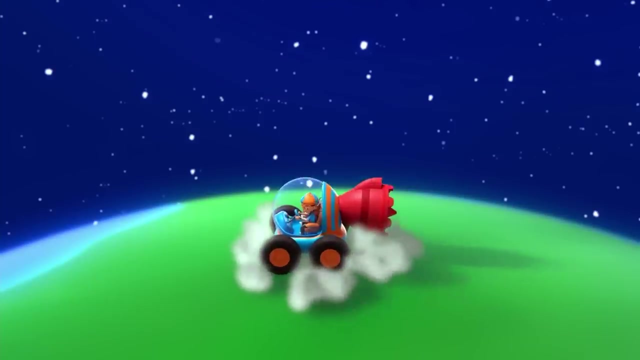 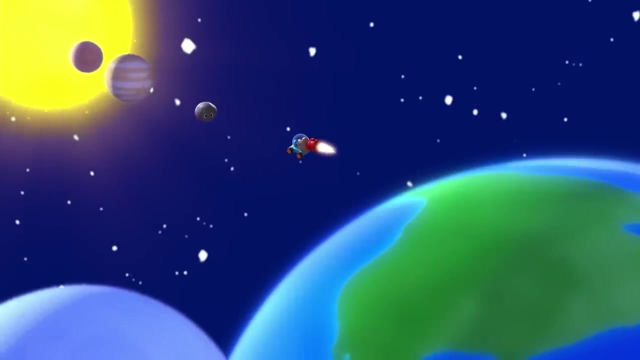 Rocket booster confirmed. Activate Blippi Station. Now it's time to get planet-sized Growing up. Ha ha ha, Right Tabs, We're in space. Whoa, It's a meteor. Hey, It's me Blippi. 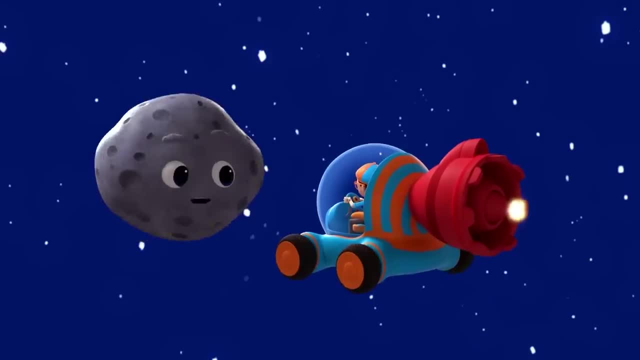 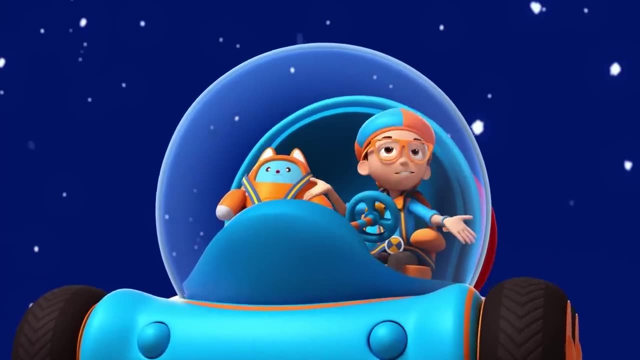 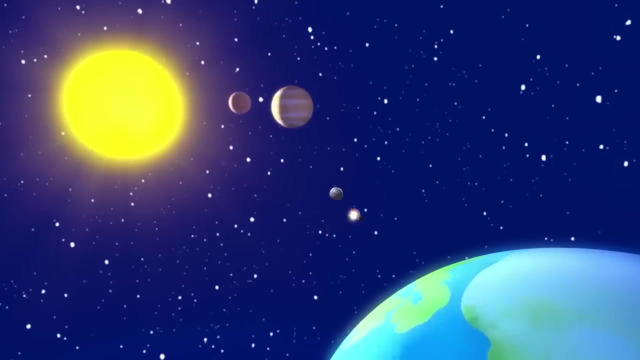 Welcome to outer space. I'm Mary the Meteor. I'm here to find out about all the planets in our solar system. There are eight planets in our solar system. Let's meet them, shall we? Closest to the blazing sun are the two smallest and hottest planets, Mercury and Venus. 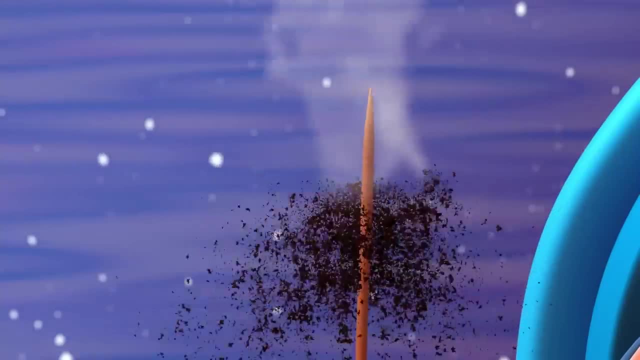 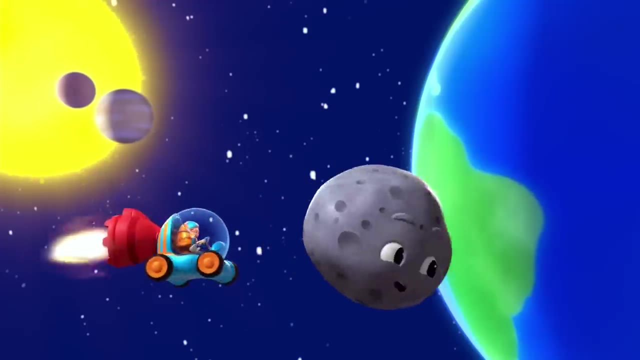 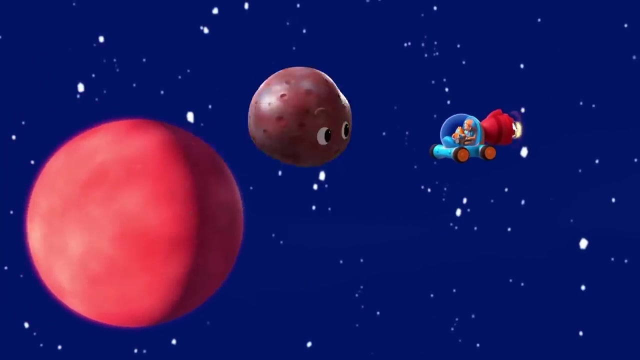 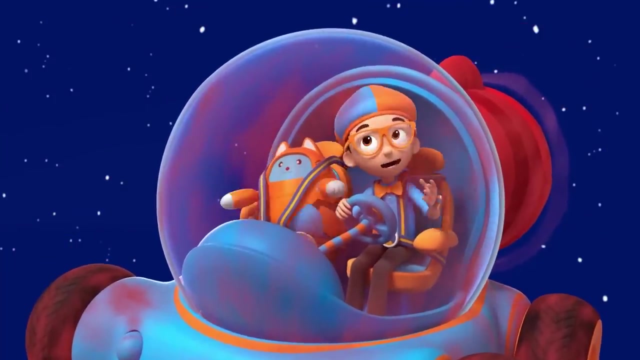 Whoa, That is hot. We should go. The third planet is your home Earth, Hi, Mom. Then there's Mars, the red planet. Mars is red because it's covered in rusty soil. Achoo, That's a lot of dust. 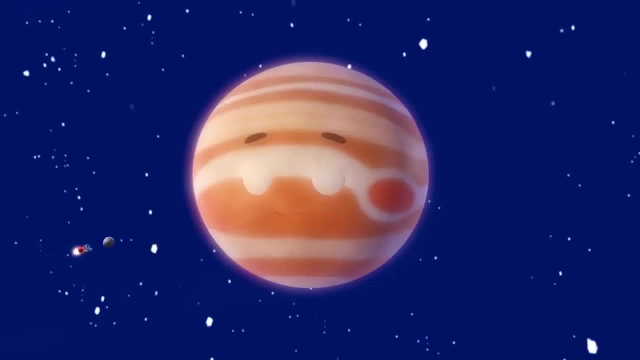 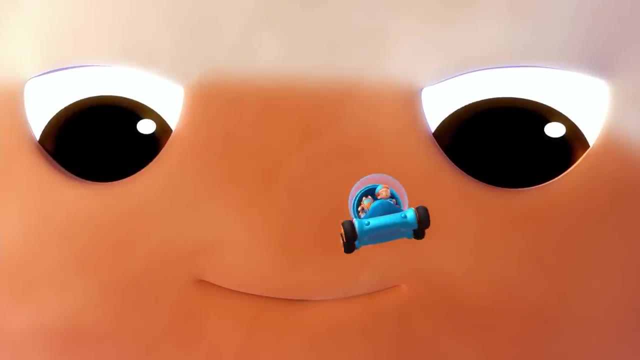 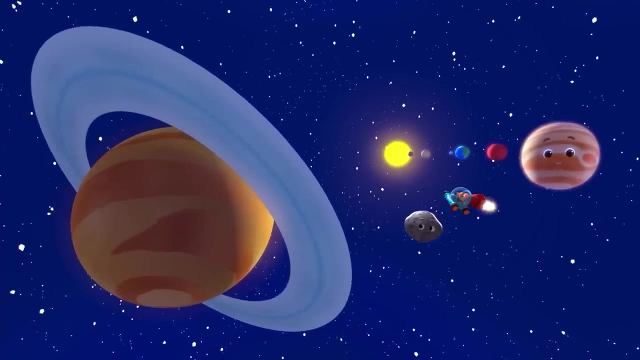 Come on. Next up is the giant Jupiter, bigger than all the planets combined. He doesn't scare me, though. Whoa, We should go. We sure are a long way from the sun now. Welcome to Saturn and her rings. Whoa, They look beautiful. 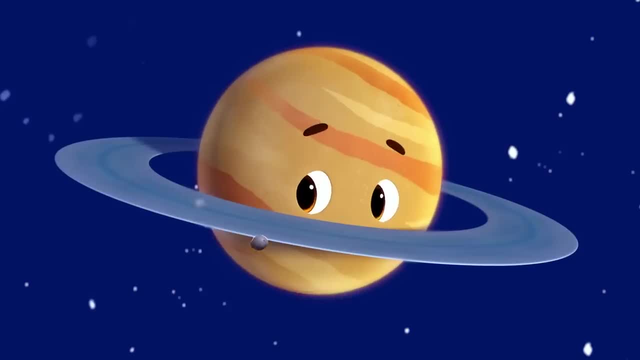 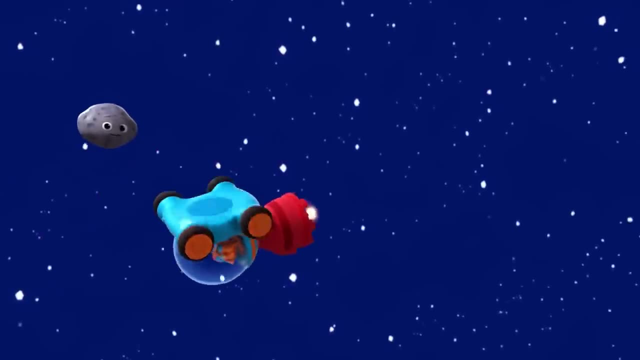 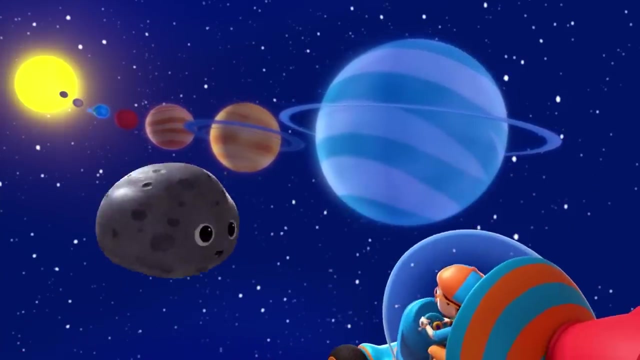 Can we get closer? Of course, Whoa, Yeah, Wee. Wait, We haven't finished yet. On your left is Uranus, billions of miles from the sun, pretty cold. Now let's hear it for the furthest. 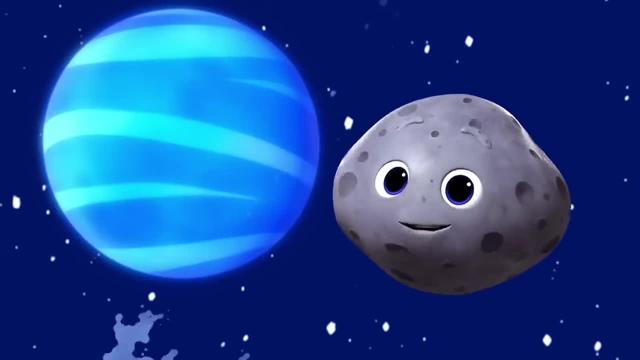 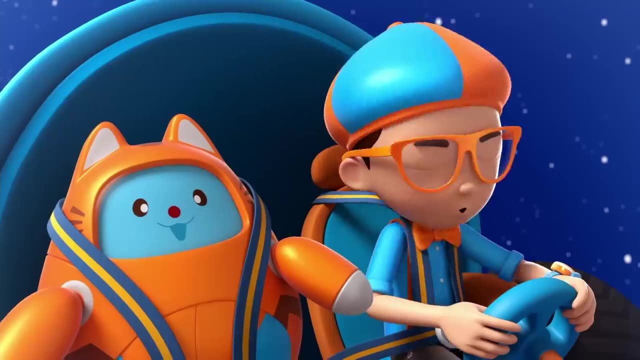 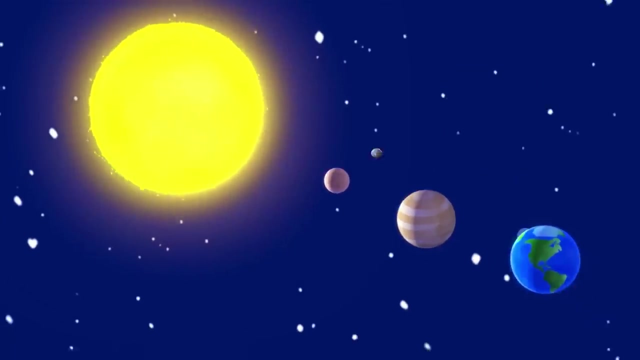 Let's hear it for the furthest, windiest and coldest planet: Neptune. Whoa, I have the answer to my question. What planets are in our solar system? Mercury, Venus, Earth, Mars, Jupiter, Saturn, Uranus and Neptune? 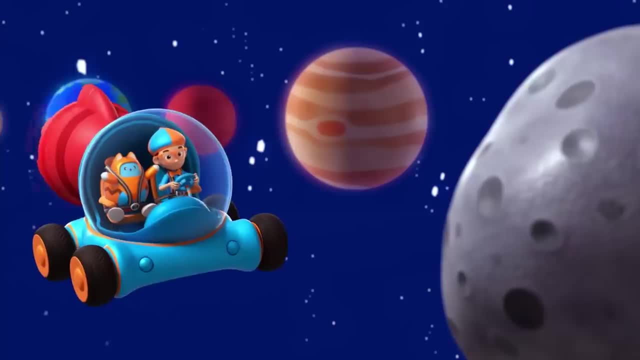 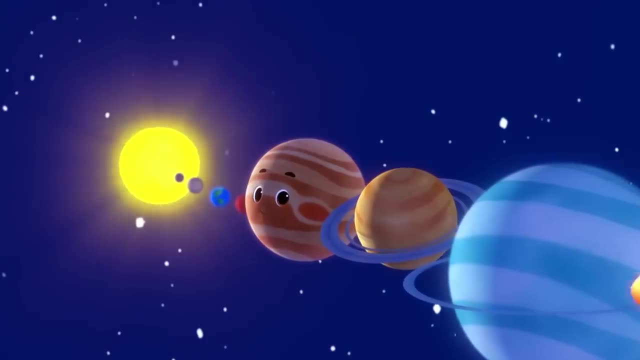 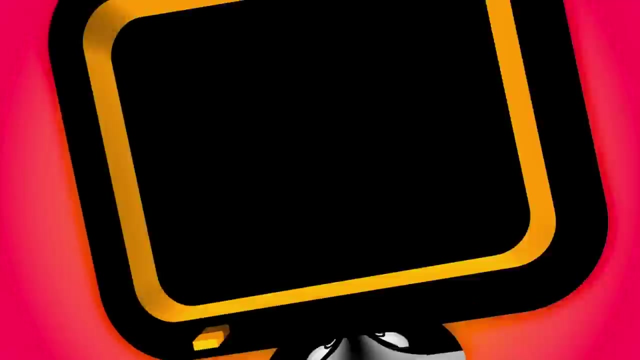 Upload answer tabs. Thanks for the tour, Mary. That was wild. See ya Blippi. Time for a shower, A meteor shower. Bye, Mary, the meteor. So much to learn about. it'll make you want to shout Blippi. 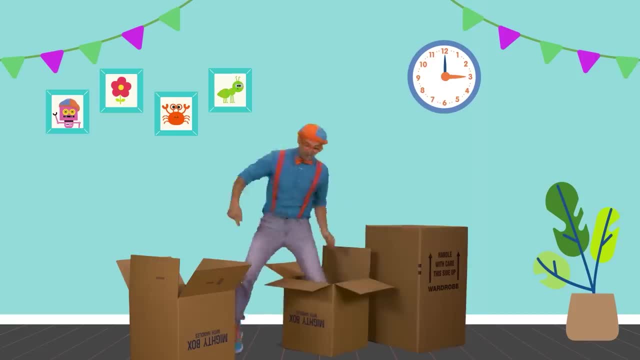 Hey, It's me Blippi, And I was just hanging out in this cardboard box. Check it out. Wee, Wee, Wee, It's like a bird Wee. I have so many cardboard boxes around here. 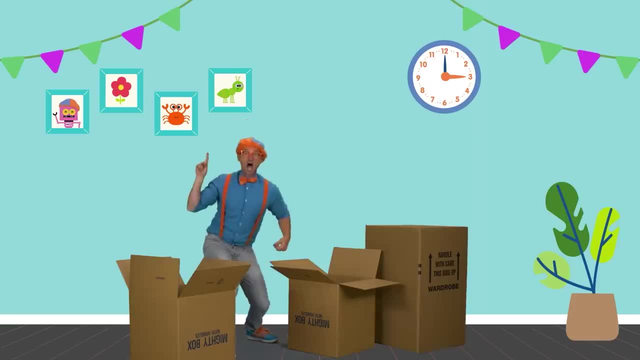 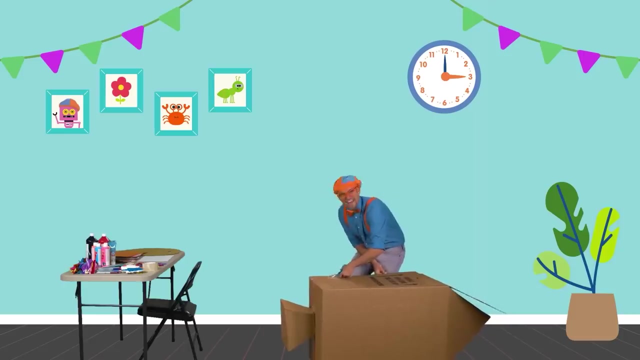 What are we to do with them? I have an idea. Why don't we take a few of these cardboard boxes and make something out of them? This is going to be fun. Oh Hey, How are you doing? I'm just making a rocket ship. 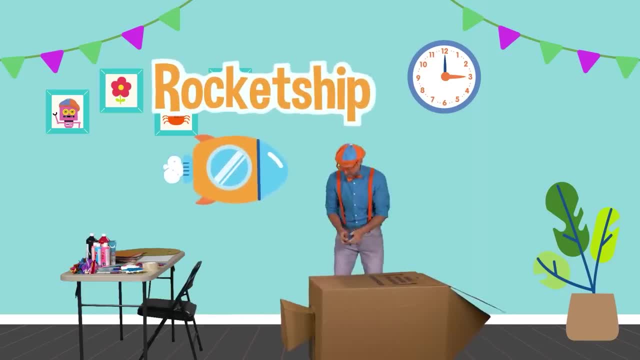 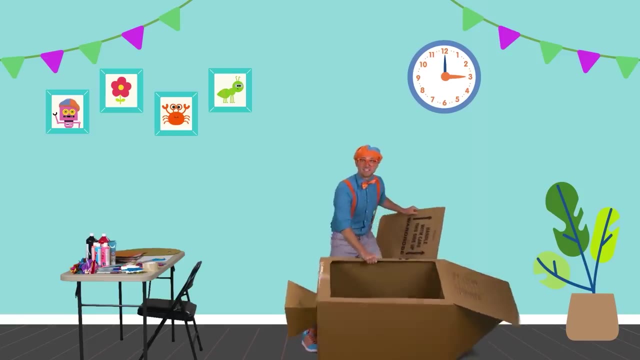 Just making a rocket ship out of these cardboard boxes. I am using these scissors, nice and safely, to cut a giant window out of it. Whoa, Look at that. Wow, Ooh, Now I can sit inside it later. Then we can explore outer space. 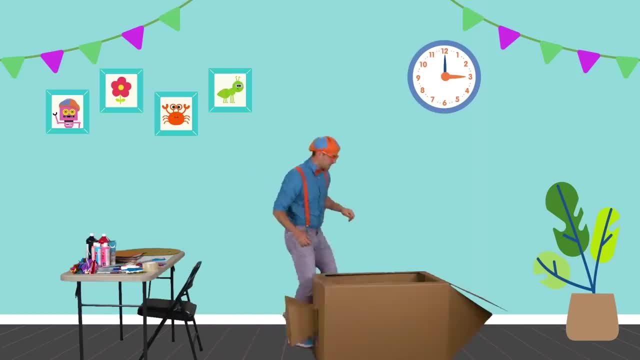 I am so excited. Okay, here we go. So, now that I have my window, I can then put the cardboard box- well, it used to be a box, now it's a rocket ship up, And do you see this? 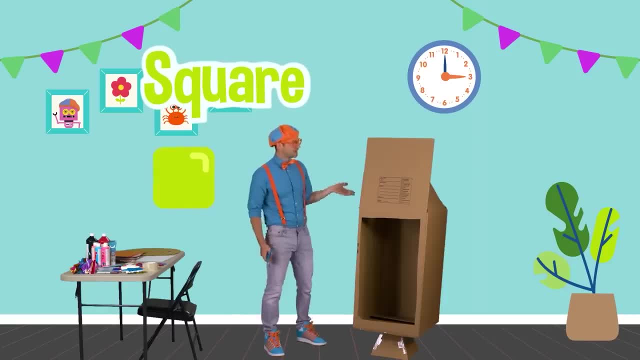 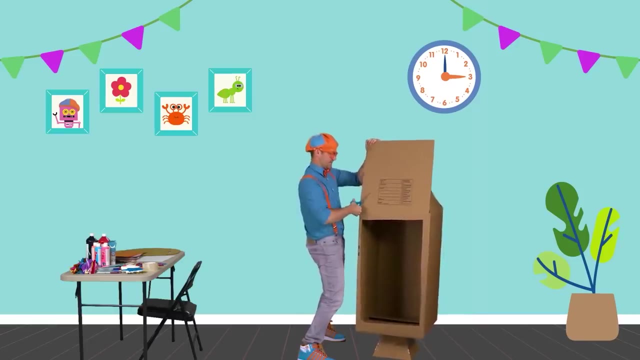 This is a square, Yeah, But we actually need to make it a triangle. So let's take our scissors. Yup, With your parents' grown-up supervision, you can cut this nice and carefully. Oh Okay, One side is done. 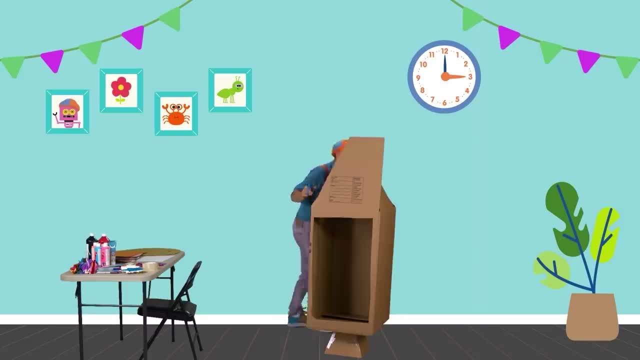 Now we need to do the other side. Here we go. Oh, Look at that, It used to be a square, but now it's a triangle, Hehe, Okay, now we need some tape to then tape it to make the top of the rocket ship. 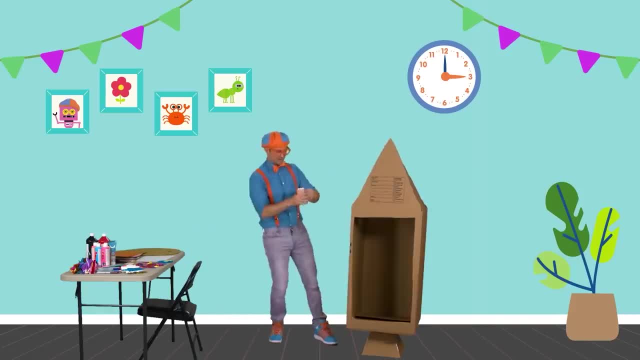 Okay, here we go. Let's grab the tape, Pull off a big piece of tape, Whoa, Alright, Let's give it a little slice. Okay, There we go. Whoa, Okay, Put that there. I love making things out of cardboard boxes. 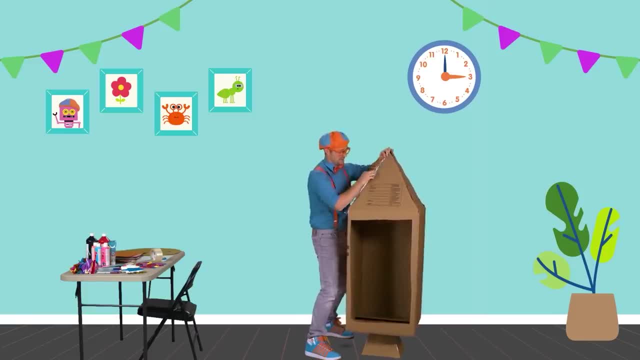 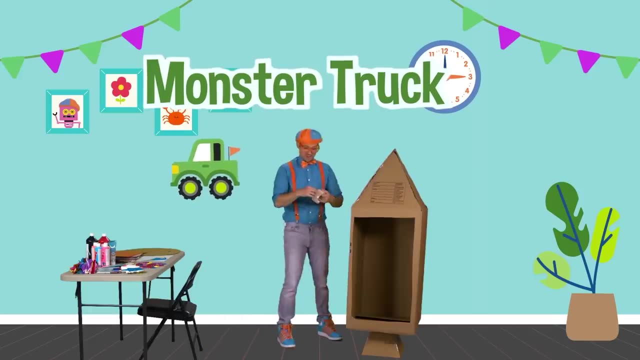 You can make so many things. Today we're making a rocket ship, But one time I made a monster truck, Another time I made a dolphin, Hehe, And I named that dolphin. Uh, what was that name? I think it was Dolphy. 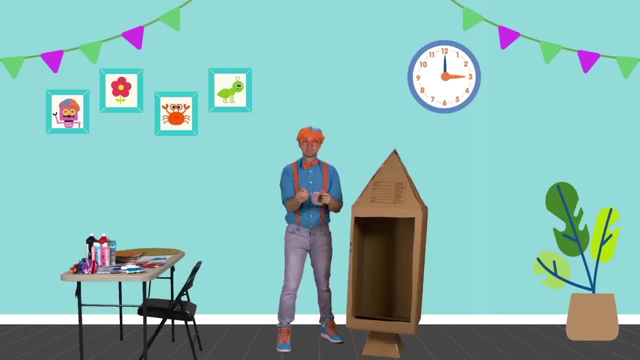 Hehe, Whoa, Sometimes the tape gets stuck, but that's okay, We got it. Alright, There we go. Give it a little slice And then tape up the other side. Wow, Here we go. I am so excited to go into outer space. 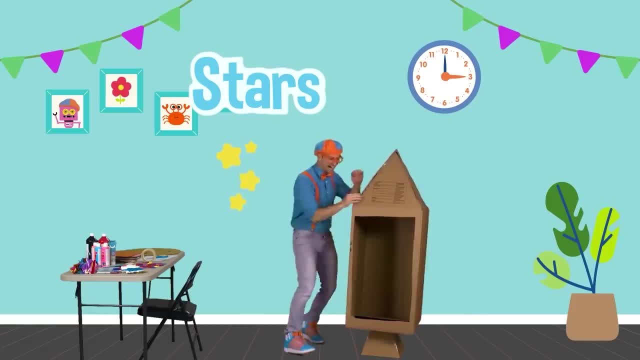 Have you ever seen the stars at night? Yeah, They're so bright. Hehe, And the moon. I love the moon. Have you noticed that the moon sometimes is a full moon or a half moon? Yeah, Sometimes it's a half moon. 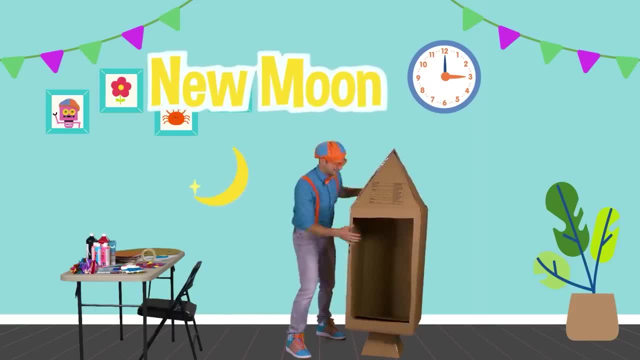 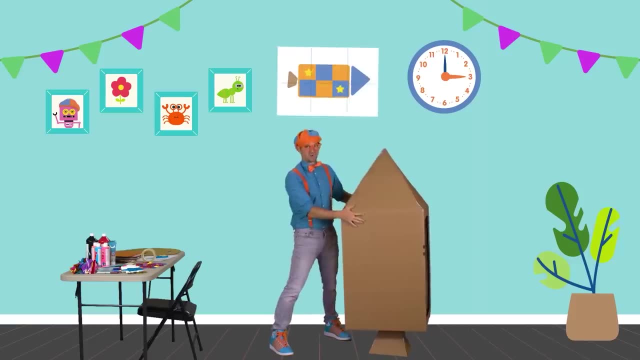 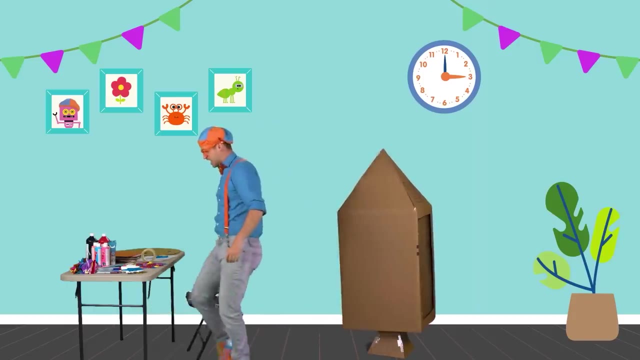 and sometimes it's a new moon. Yeah, Okay, Let's uh give this a little twist and now it's time to design our rocket ship. I am so excited. This is one of my favorite parts. So the first step to design. 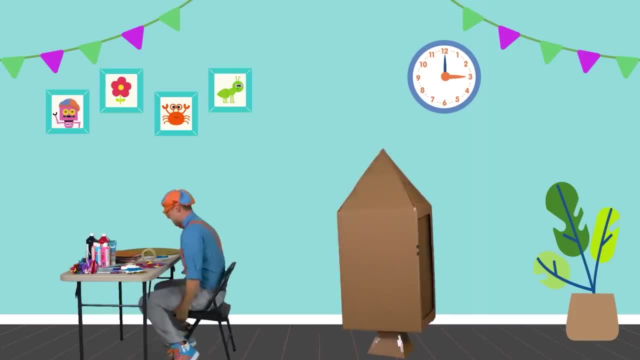 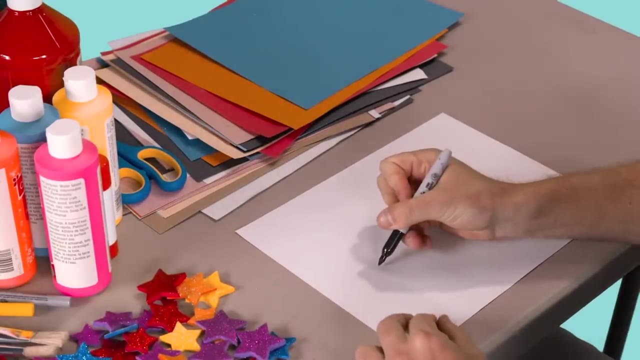 is to have a plan. So let's take this white piece of paper right here and let's draw the rocket ship. So the first thing you need to do is plan, Plan how the rocket ship is gonna look. So let's draw the rocket ship. 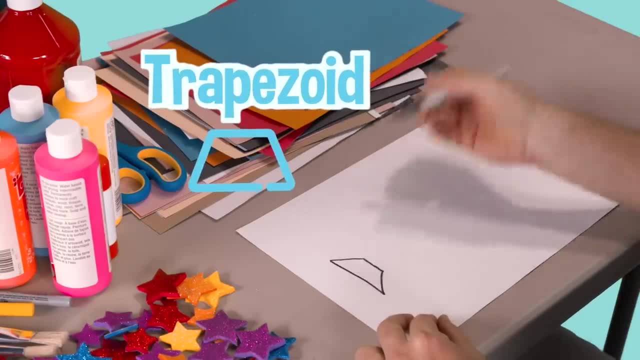 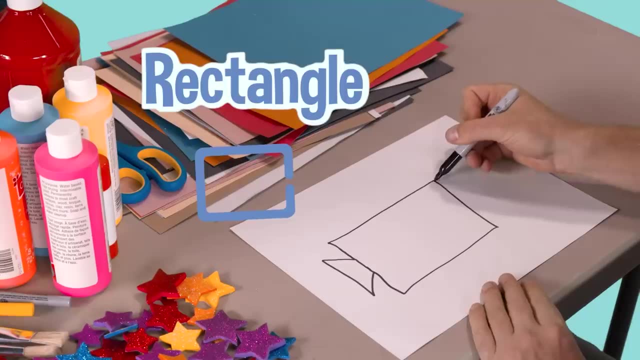 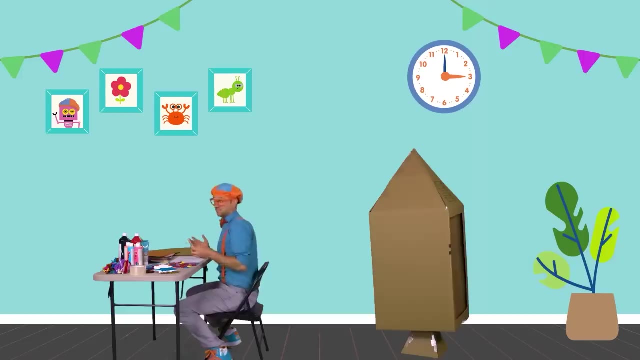 So we have a trapezoid over here and then we have a big rectangle for the body of the rocket ship, and then we have a triangle for the cone of the rocket ship, And obviously I want a lot of color. 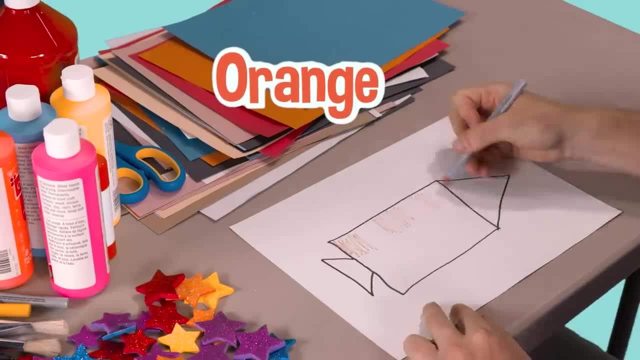 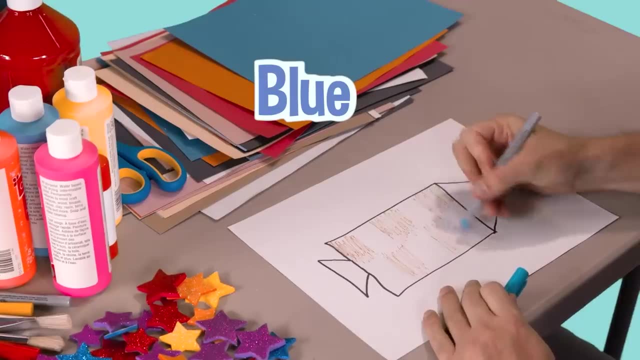 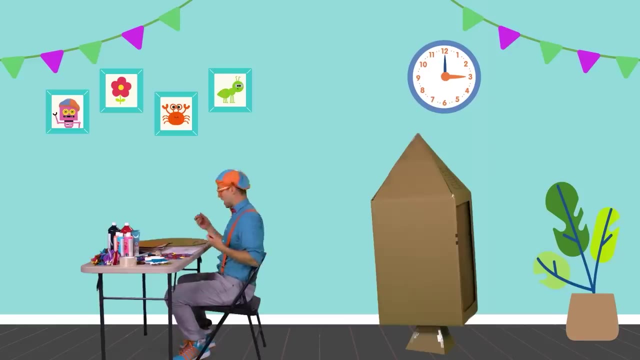 So first let's take some orange- Perfect, I love orange. Then let's take some blue. So let's color it in. I have a plan: I'm gonna use colored paper for that, So I'm actually gonna use this black marker. 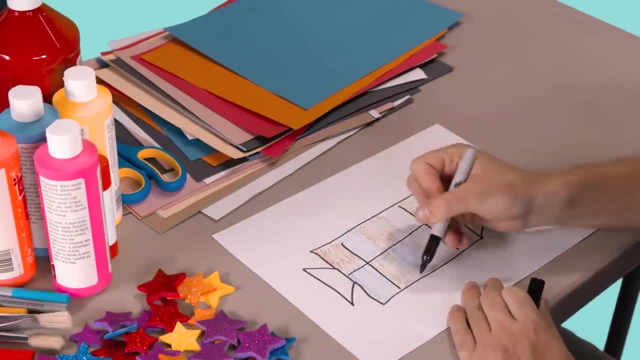 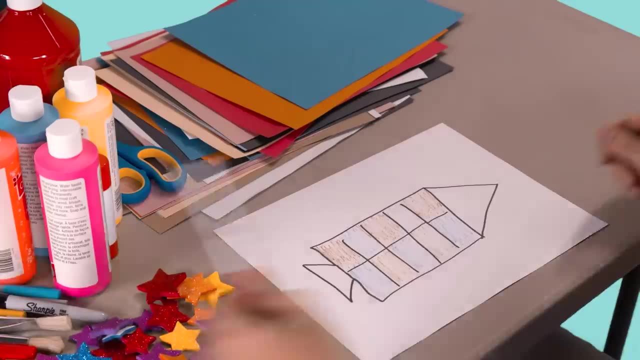 to symbolize that these are pieces of paper And we do that later. Alright, Oh, whoa, There's a lot of stars here, So let's actually, you know, make some stars right here. Yeah, Yeah. 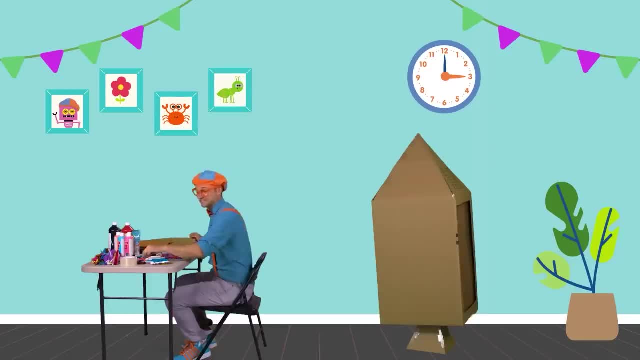 I love stars Because you see them at nighttime, when you look up in the sky and they twinkle, Yeah, kinda like Twinkle, twinkle little star. how I wonder what you are. You know that song. 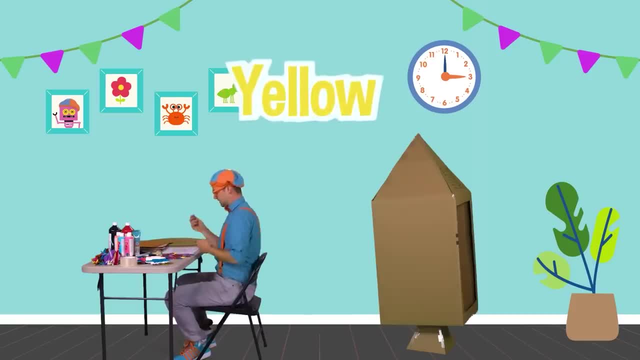 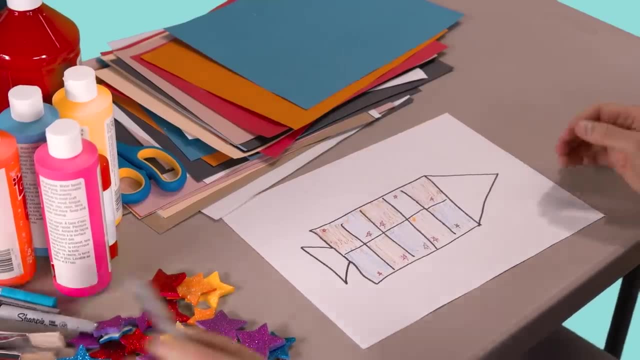 I like that song too. Ooh and yellow- Yeah, that's a beautiful color. Wow, Our rocket ship is looking so good. Alright, I think I have a really good idea. Let's take the color red, because it's nice and bright. 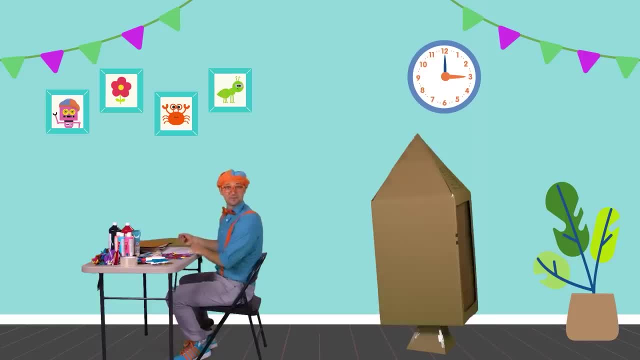 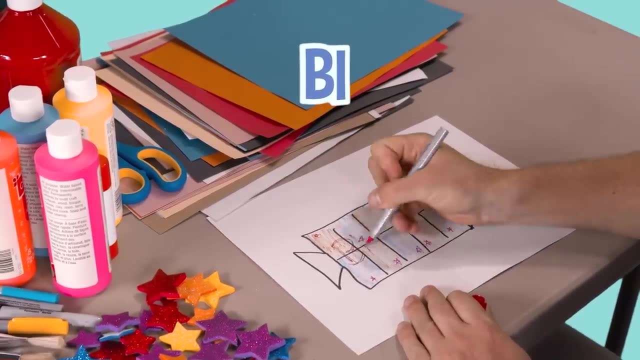 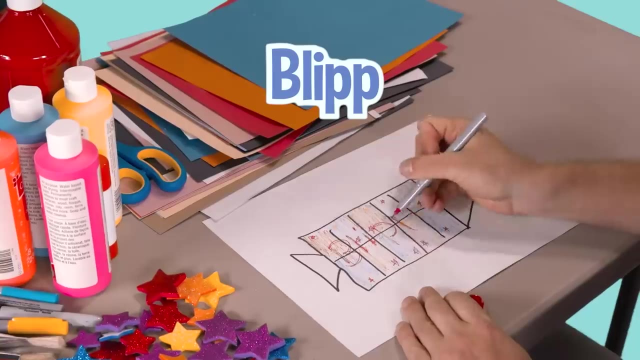 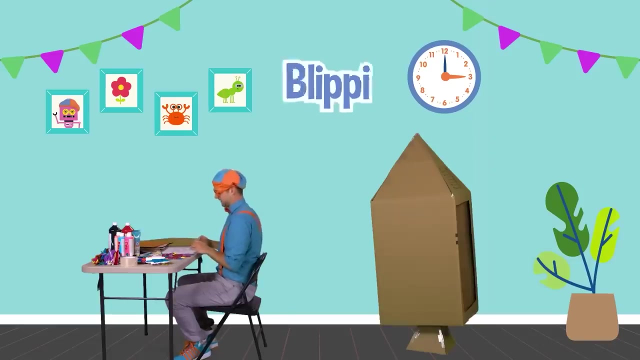 and spell my name. Will you spell my name with me? Ready, B, L, I, P, P. Here we go. Yay, blippy, Perfect, Alright, so that is the plan. Oh, Looks like this triangle, the top of the rocket ship. 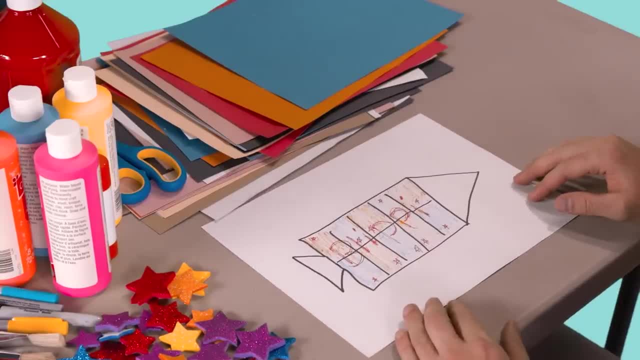 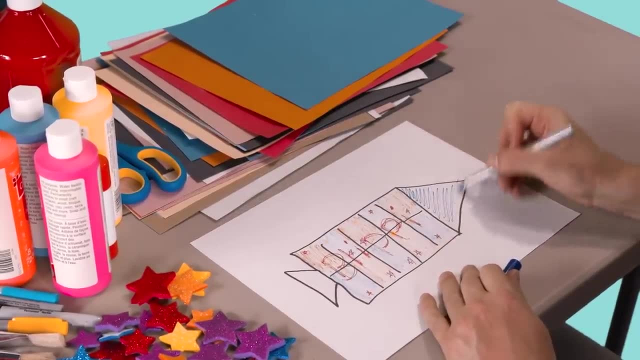 Yeah, we could color in. How about we color it? yeah, Blue, I like blue And we actually have a lot of blue paint on the here is, so we can actually just use blue paint for this part. Wow. 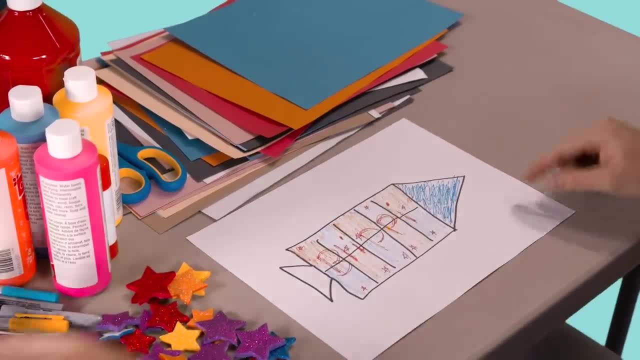 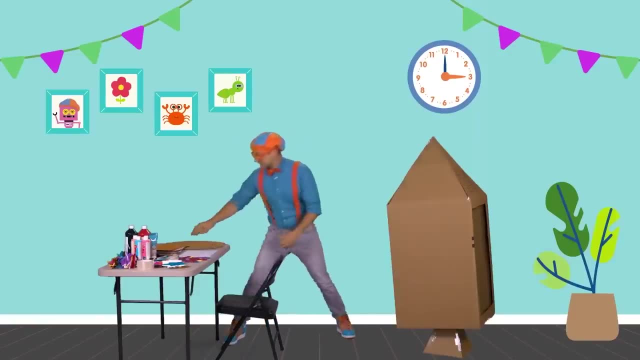 Wow, I think if we can make this rocket ship in real life, it's going to be so good. All right, here we go. All right, like I said, first thing we have to do is use the blue and orange colored paper. 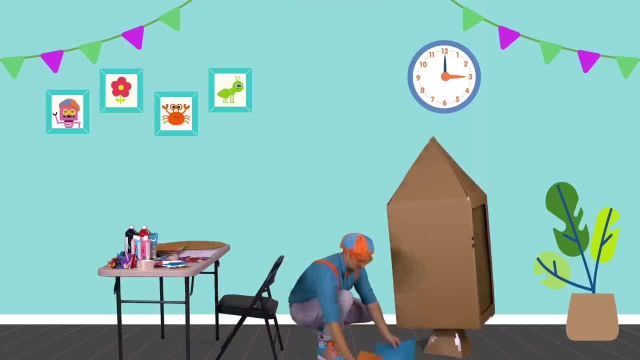 to put on the side, just like this. So let's take the glue stick. yeah, yep, put a lot of glue right on the backs, Just like that. okay, there's two pieces. okay, there's one, and here's the second piece. 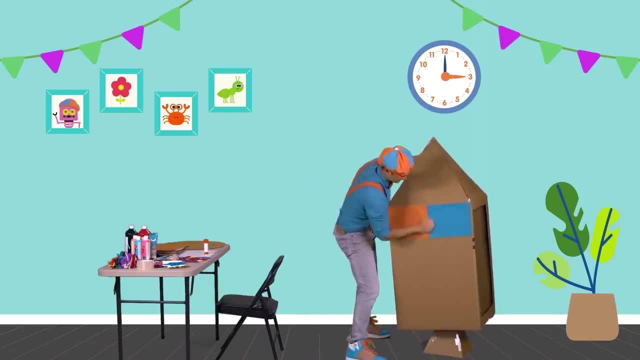 All right, there's one, two pieces of paper and we've got one, two, three, four, five, and let's do two more, yeah, which will make one, two, three, four pieces of paper. I'm going to put the glue on them right over here. 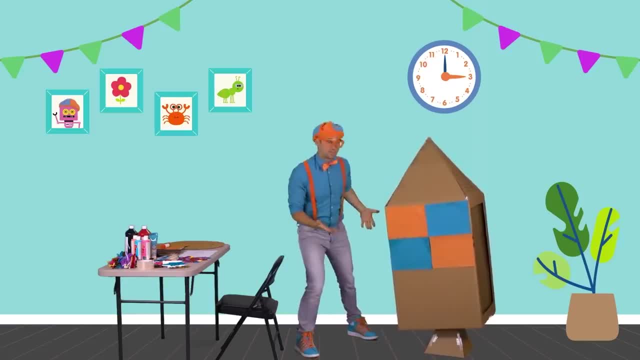 Okay, now we have four pieces: one, two, three, four. So let me finish the rest and then we'll see how many we have in total after I'm all done. all right, Whoa, it's falling apart. well, sometimes, if things fall apart, you just have to fix. 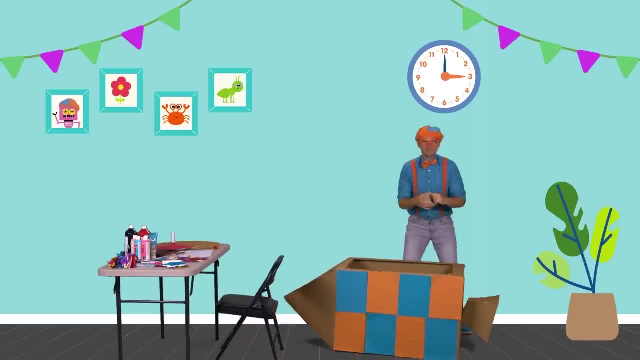 them. Okay, here we go. and after we fix this, then we can count all of the colors. so let's take our tape. All right, here we go. Okay, now the rocket booster is all fixed. Yep, there we go. 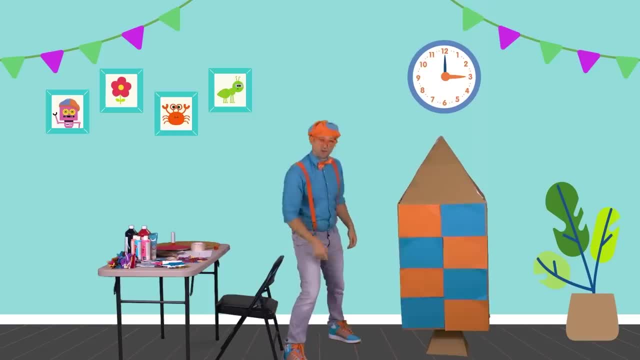 Okay, now let's count all of the colored pieces. yeah, the blue and the orange pieces, Those are my two favorite colors. Okay, there's one, two, three, four, five, six, seven, eight, eight pieces of paper. 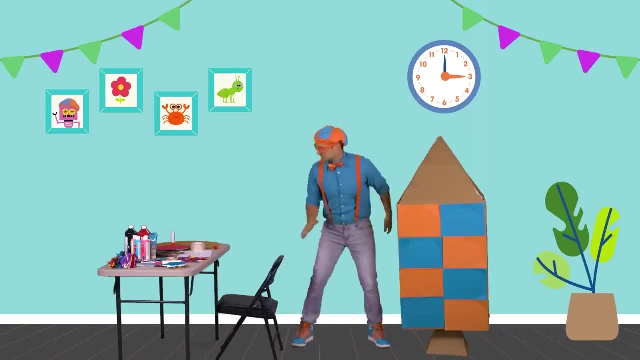 Paper. good job. Okay, what else did we have on our piece of paper over here of our initial plans of our rocket ship to go to outer space? We had stars. Yeah, remember, We had yellow stars. Yellow star, Another yellow star. 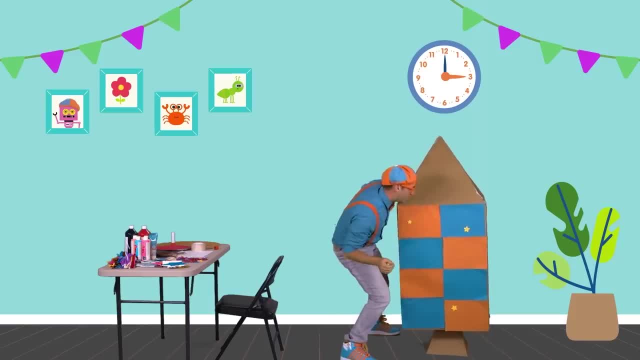 Wow, They're so bright and they twinkle just like the real thing. Okay, and let's put some blue stars on there. Can you think of anything? that's the color blue My shirt? What about the big, vast blue ocean? 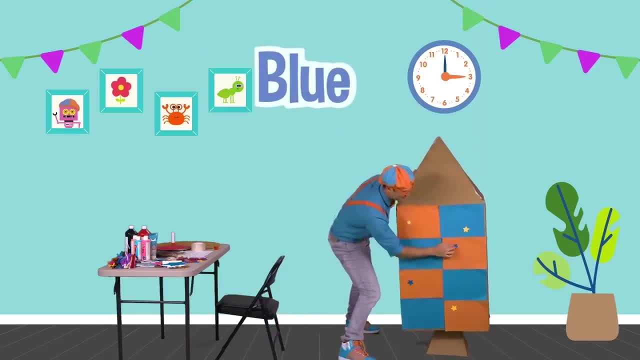 Yeah, Here's another blue star. Here we go. What about a purple star? Yeah, I like the color purple Right there. And, last but not least, another purple star Right there. Perfect, That looks so cool, All right. 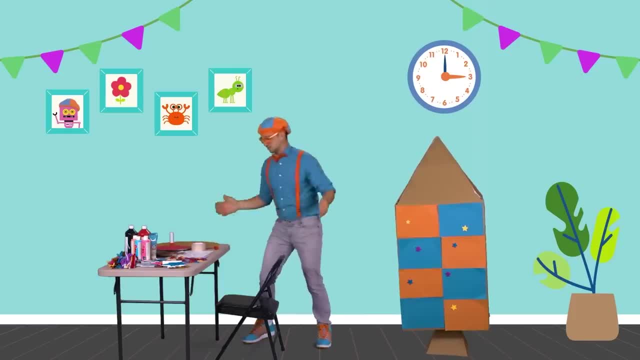 So, as you remember, we have to spell my name on it because that's what was on the plans. But before we do that, let's do the top of the rocket ship. Remember what color I said I was going to paint it? 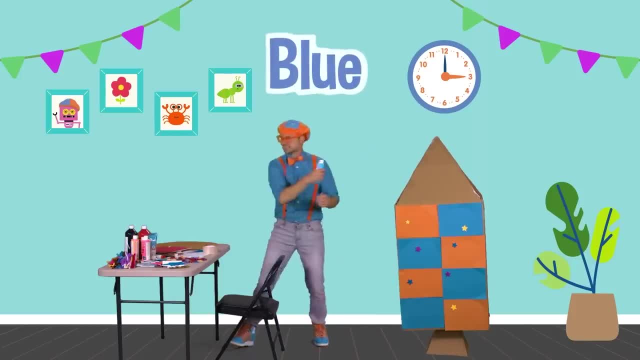 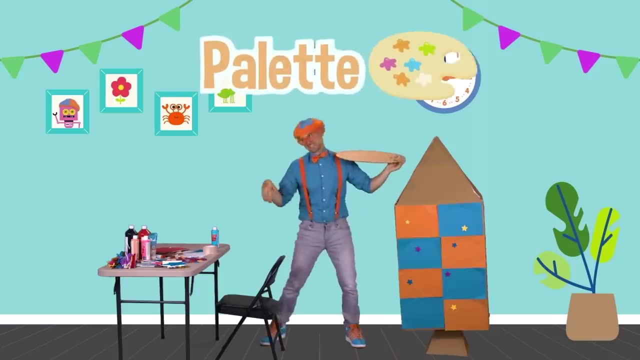 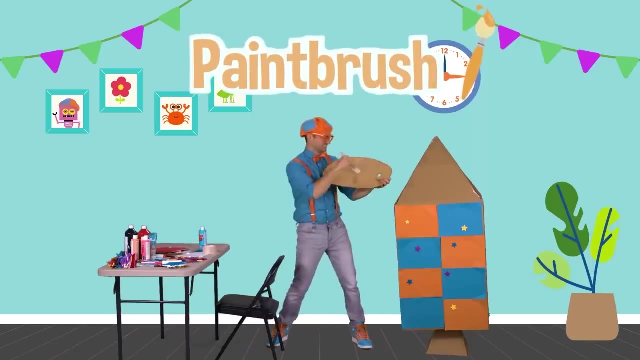 Yeah, the color blue. Okay, let's take some blue paint and my painter's palette, My painter's palette. I'm an artist. And let's take a paintbrush. Ooh, I love painting. Okay, let's squeeze some blue paint right on top. 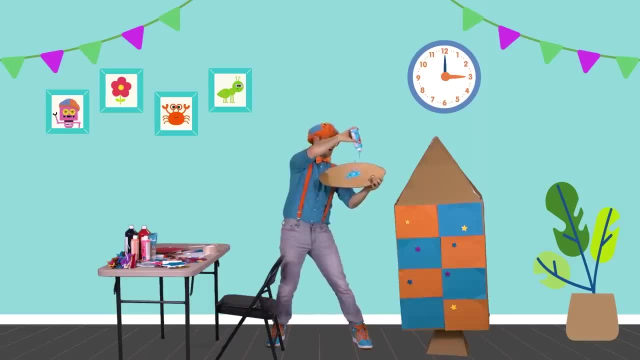 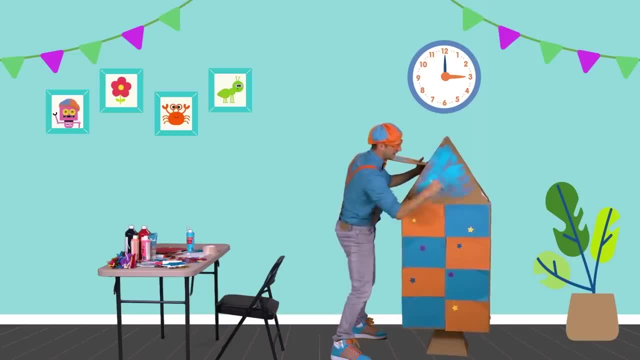 Wow, Whoa, Whoa. there we go. Have you ever used paints before? They're so fun. You can use a paintbrush and you can even use your fingers sometimes. We won't do that today, but that art technique is called finger painting. 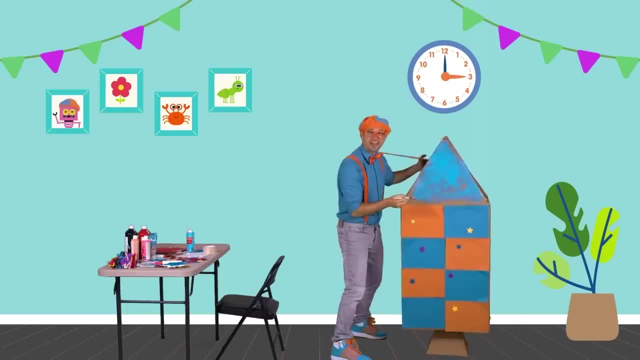 There we go. How does that look? Do you like that? Yeah, I do too. Okay, let's put this away. You need to stay nice and clean and organized. There we go, And remember the last thing we needed to do. 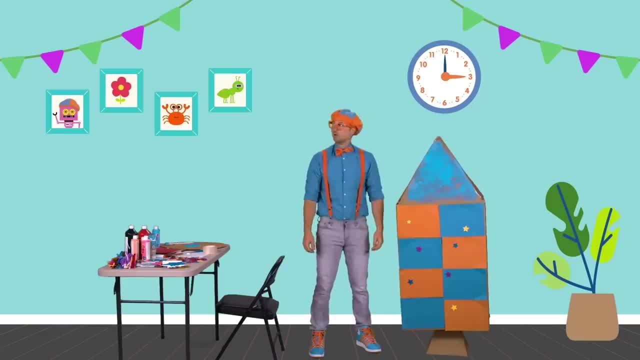 We needed to spell someone's name. Oh yeah, My name Blippi. Will you spell it with me? Blippi, Blippi, Blippi, Good job, And do you remember what color? Yeah, The color red, Okay. 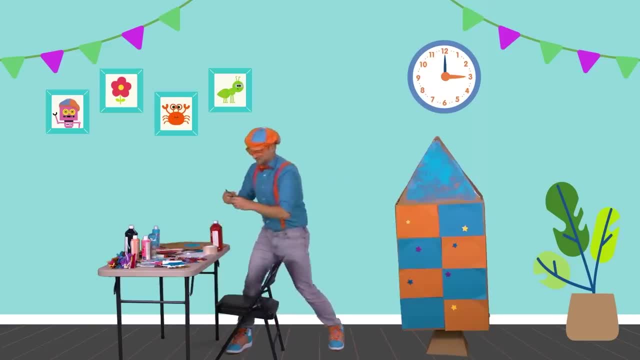 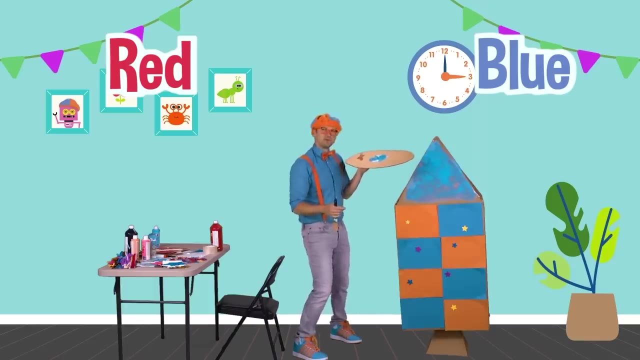 So let's use a new paintbrush, Yep. And then we need to make sure we don't mix the red and the blue, Because then it won't be red anymore And a blue, And then it won't be blue. 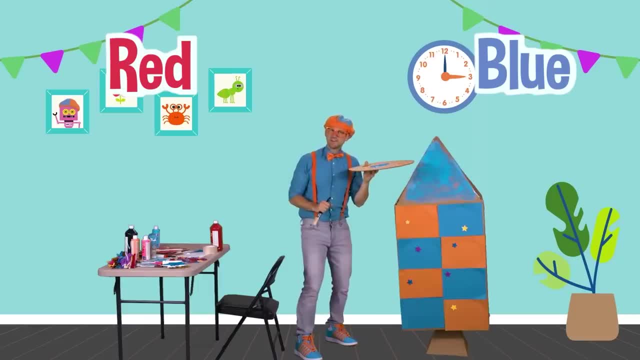 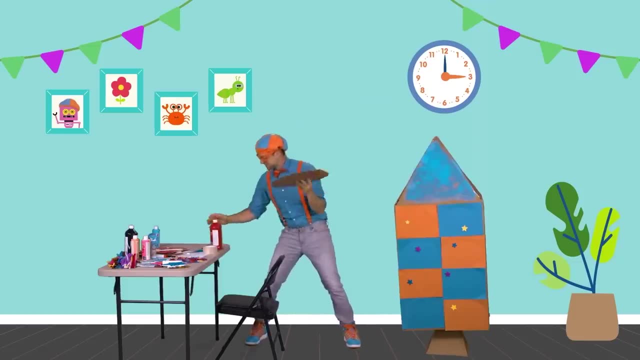 Do you know what color you get when you mix blue and red? Yep, Purple, But we're going to keep them separate, So let's take this cap off. Oh, there is so much paint in here And I like to use a lot of paint. 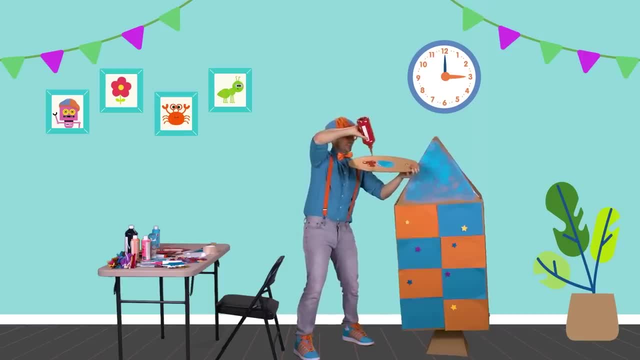 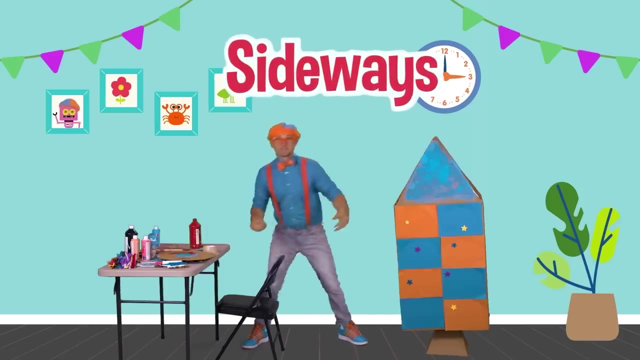 Whoa, There we go. Wee Whoa, A little bit more Boop. All right, There we go. Okay, Let's, Before we paint it, we should probably lay it down sideways, Because we need to write my name, which is sideways. 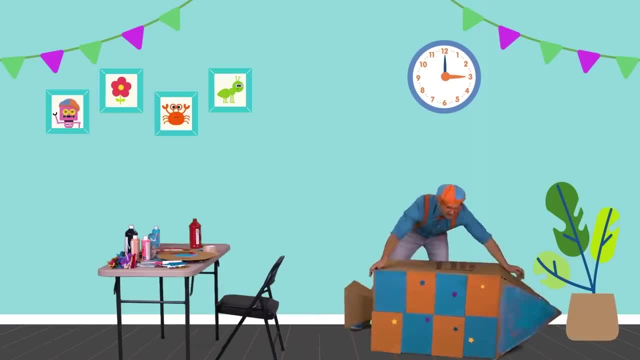 Yeah, There we go Like that. That's how we write Sideways. Okay, Let's take our paintbrush And let's put the letter B right here. All right, Now that we have the letter B. the second letter is the letter L. 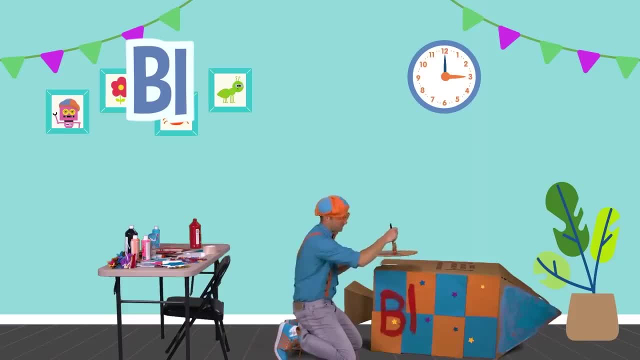 Yeah, Just like that. The third letter is an I Ready. Okay, There we go, B-L-I. You know the next letter: A P, Yeah, B-L-I-P. All right, B-L-I-P-P. Yeah. 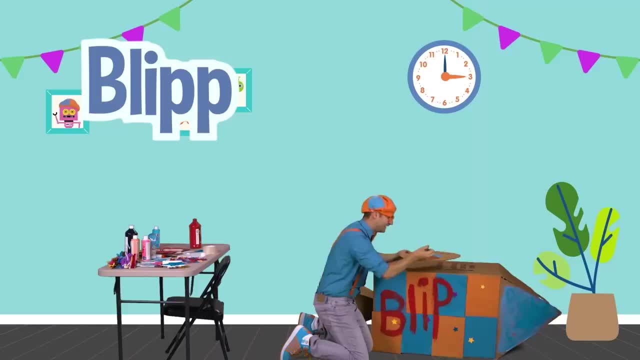 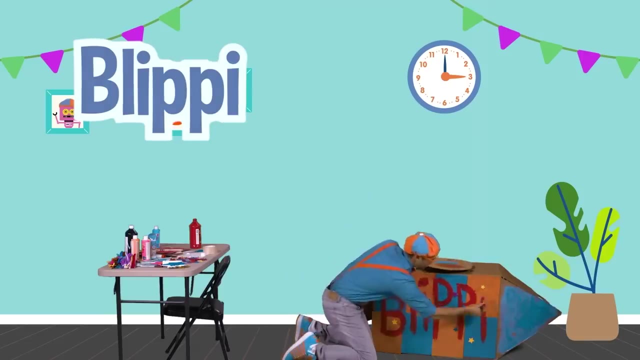 Here we go. All right, One last letter: B-L-I-P-P-I. Yes Blippi, good job, There we go. We just completed the rocket ship, So now we gotta get inside. Oh no, Do you see what I did? 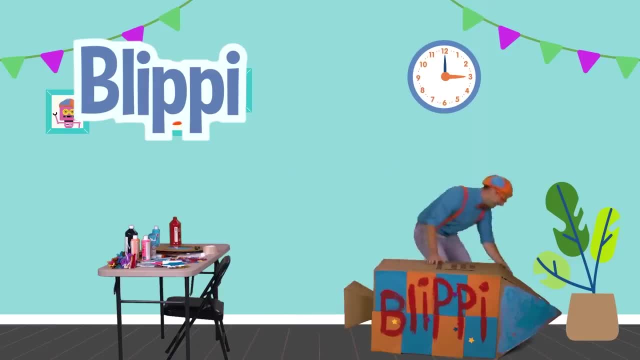 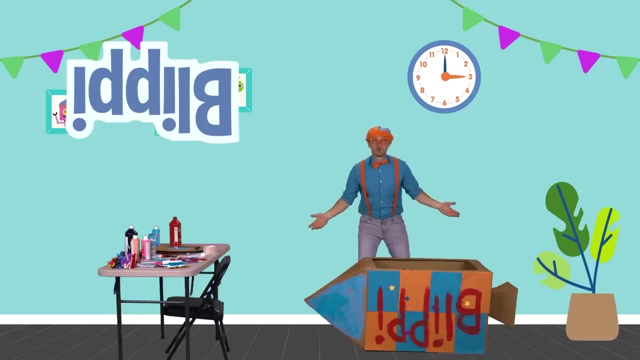 We're so silly, Check this out. The window is right there. Yeah, That means we have to twist it this way, See, And now my name is Upside Down. That's okay, though We're gonna fly through outer space in this new cardboard rocket ship. 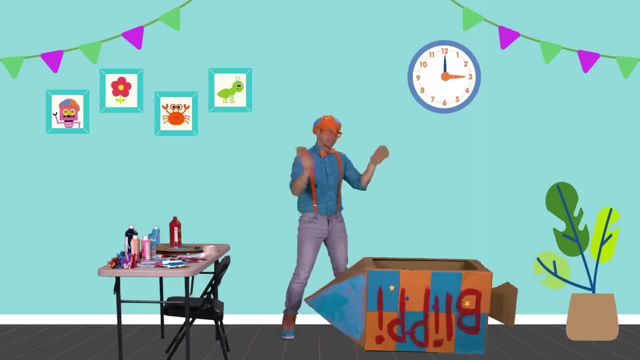 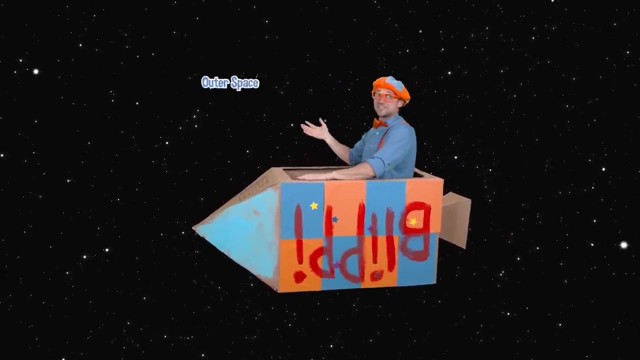 I am so excited With my name being Upside Down. So, silly, Are you ready? Ready, Because I sure am. Here we go. Hey, I love outer space. Good job building the rocket ship with me Now that we're in outer space. 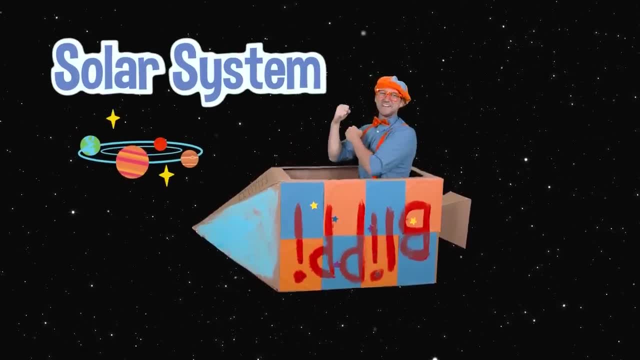 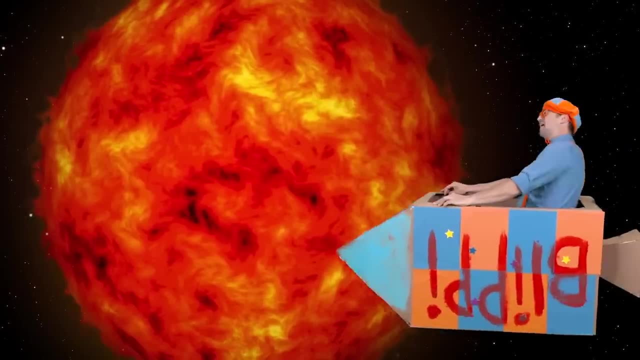 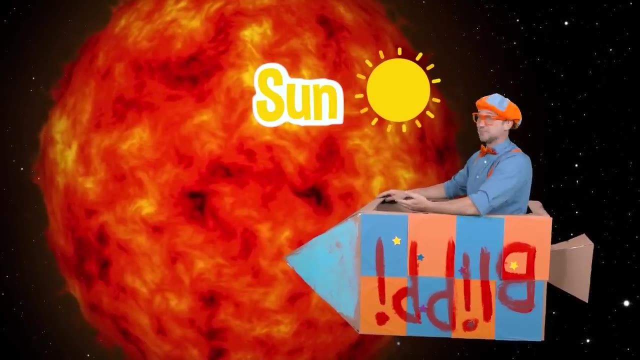 I think we should explore our solar system and learn all about it. Alright, here we go, Whoa Whoa, Whoa, Whoa Whoa. Look at that, That is our sun, And its name is called the sun. 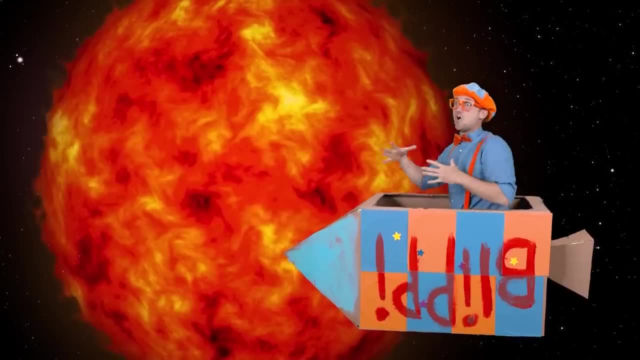 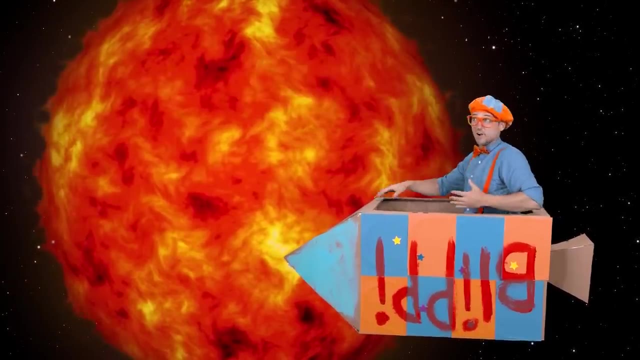 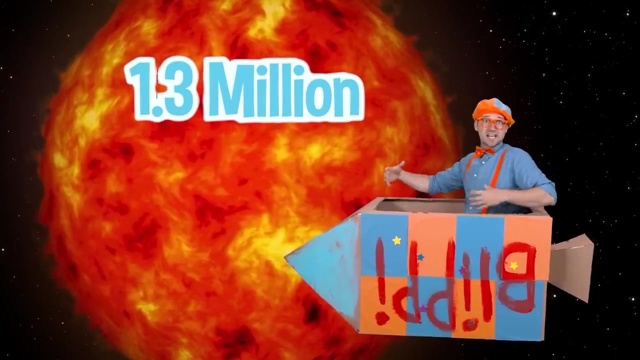 How original. Our sun provides all the light in our solar system And that light takes eight minutes to go from the sun to our planet Earth. And the sun is so big: there's 1.3 million Earths that can fit inside of it. 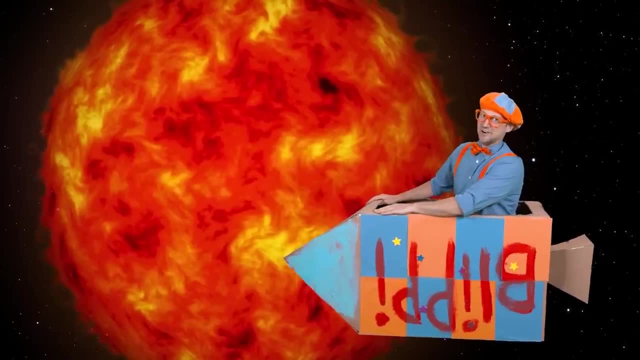 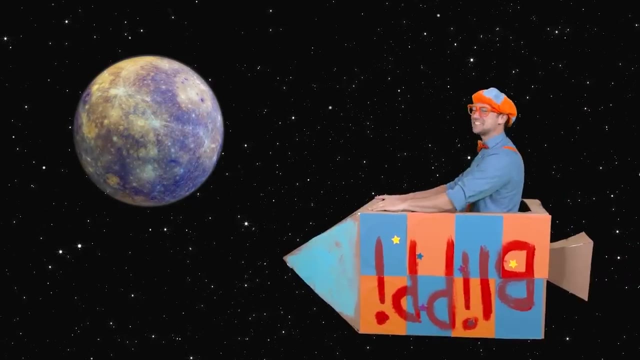 Whoa, Whoa, Whoa, Whoa, Whoa, Whoa, Whoa. That's a lot of Earths. Here we go. Woohoo, Ready Whoa. Outer space is so much fun Oh. 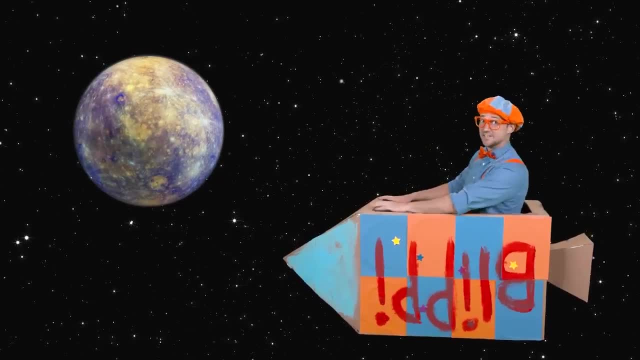 Look at that planet. That planet is Mercury. Wow, That planet is really rocky And there's so many craters on it And actually, since it's the closest planet to the sun, one rotation around the sun, it's going to be the closest planet to the sun. 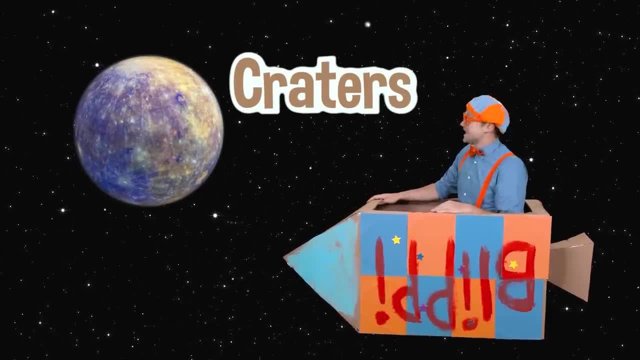 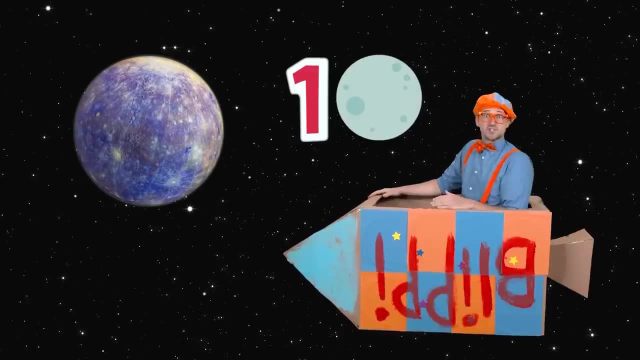 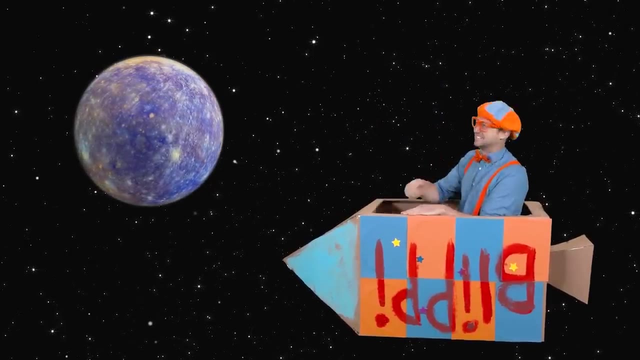 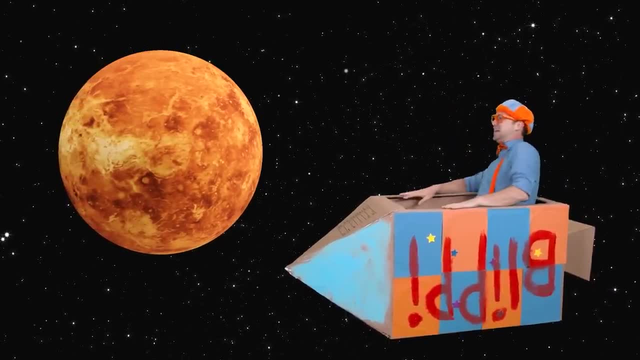 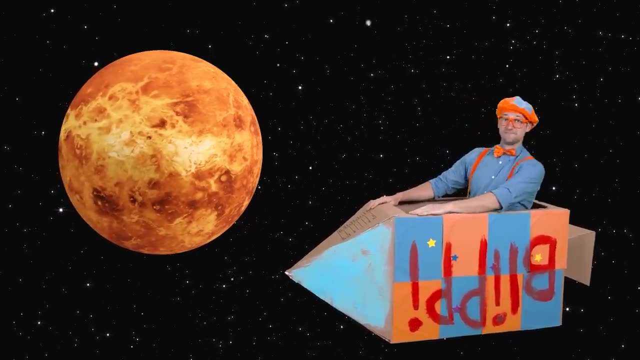 Woohoo, Woohoo, Ha, Yeah, Whoho. Now we're at another planet. Look at that planet. That planet is the planet Venus and it is so hot, It's the hottest planet. Woo, It's getting hot in here. 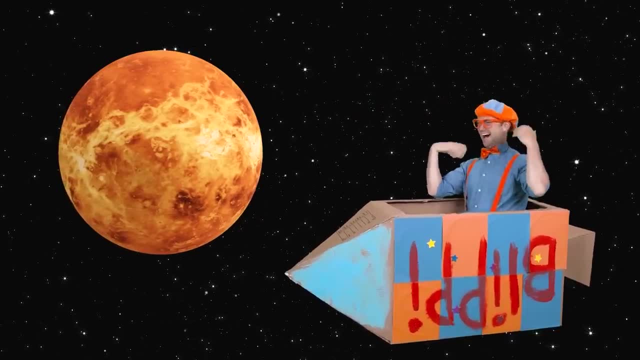 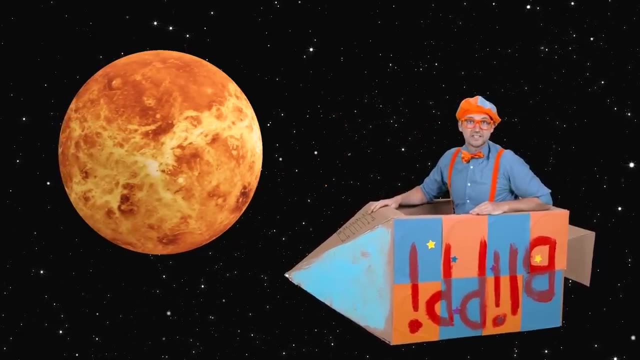 Haha, The planet is so hot. It's getting hot in here. Haha, The planet has so many volcanoes on it And it's actually really bright. If you look up in the sky from our planet Earth, you can actually see it without a telescope. 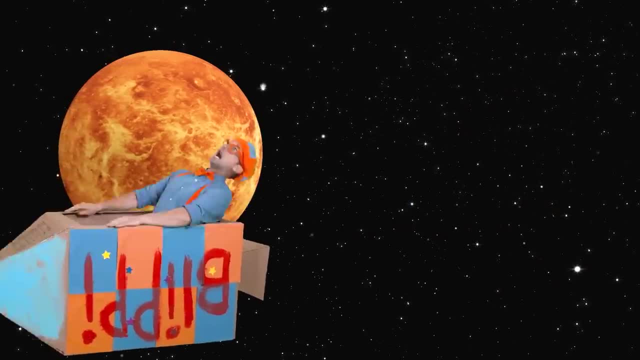 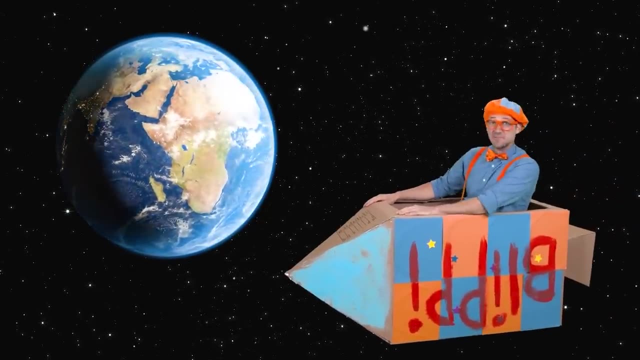 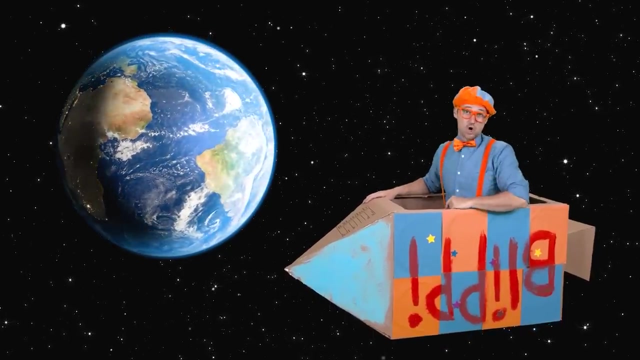 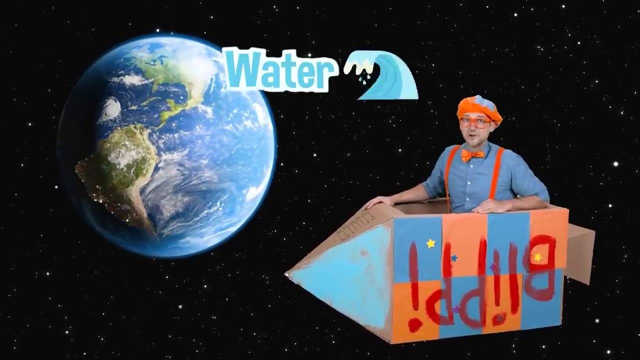 Wow, Here we go. This has been awesome. Whoa, Is that you right there? I think I see you. Hey, that's planet Earth. That's where you and I live. Wow, what a beautiful planet. There's so much water there. 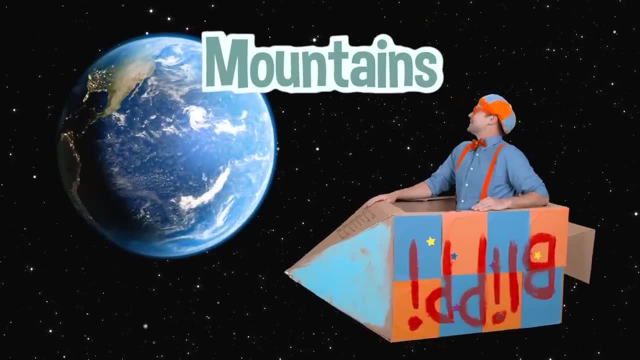 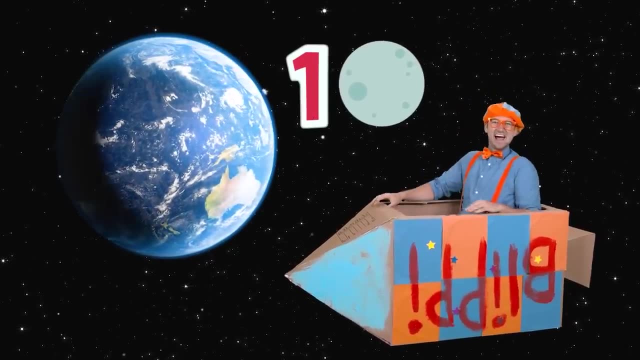 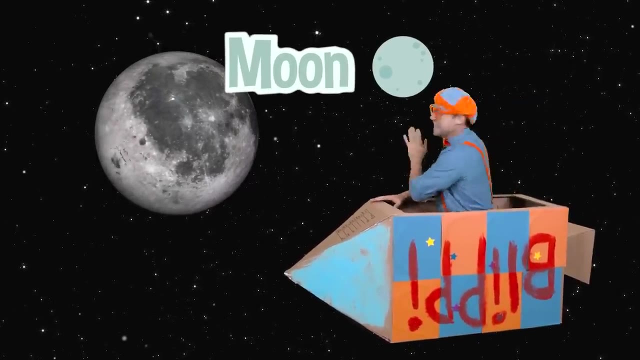 And then there's a lot of trees and mountains, Whoa, And our planet Earth. yeah, we have one moon. Let's head there now. Woohoo, Woohoo, Whee, Hey moon. Thank you so much for lighting us up. 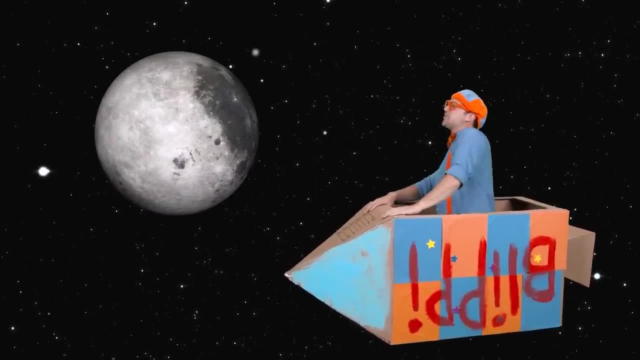 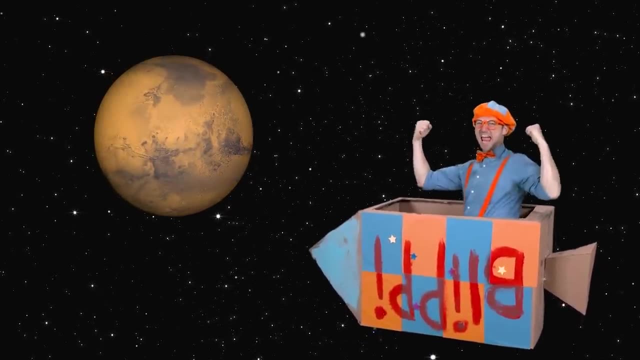 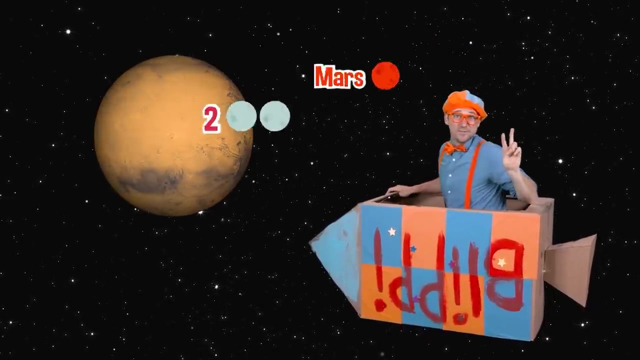 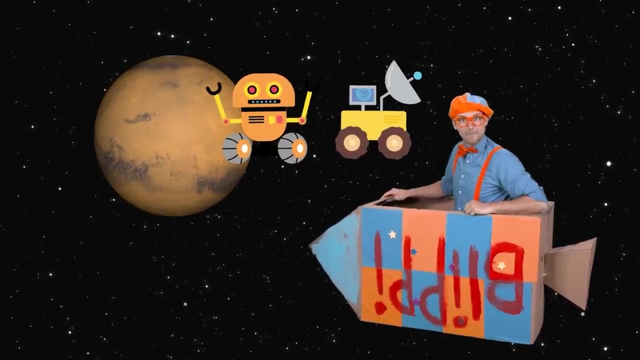 at night: Woohoo, Whee, Woohoo, Woohoo. Another planet, Yeah, Ooh, that planet is the planet Mars. Whoa, it has two moons. Wow, what a lucky planet. Well, we've actually sent robots and rovers to Mars. 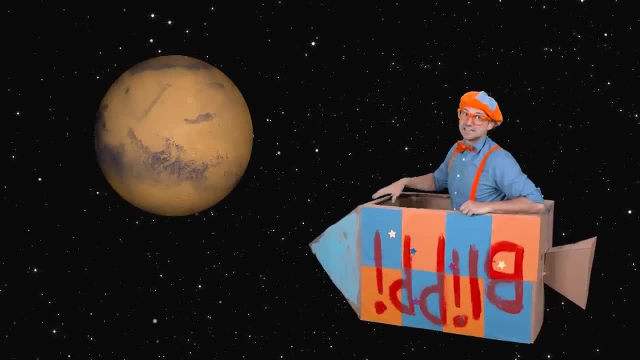 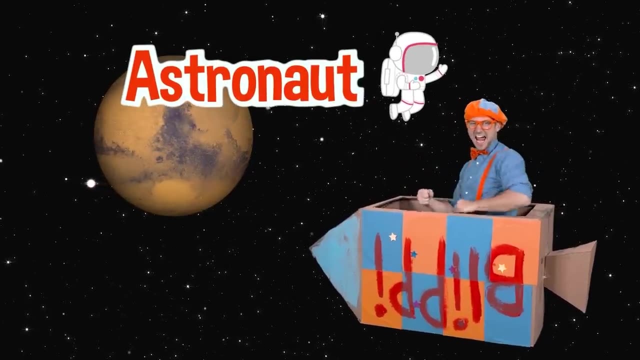 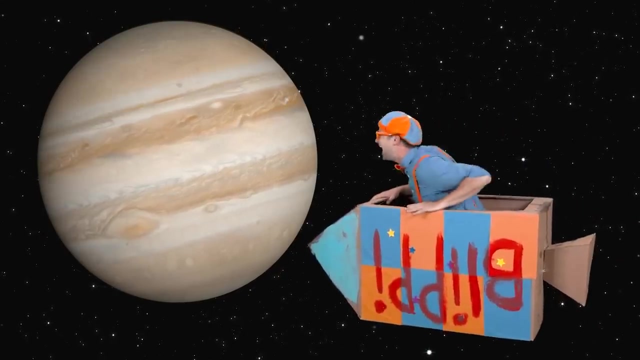 That is awesome. Us humans have yet to land on Mars, but maybe someday soon, maybe you'll be that astronaut. Yeah, Here we go, Woohoo, Woohoo, Whoa. Haha, That asteroid belt was so intense. 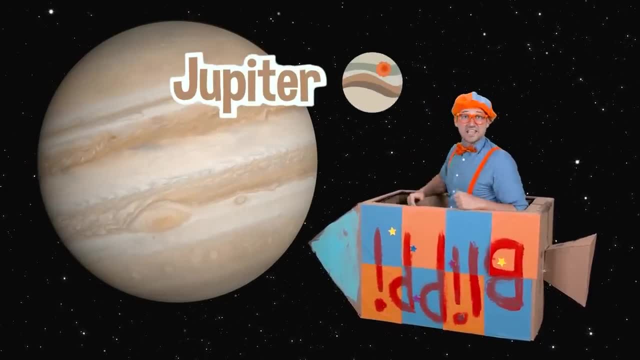 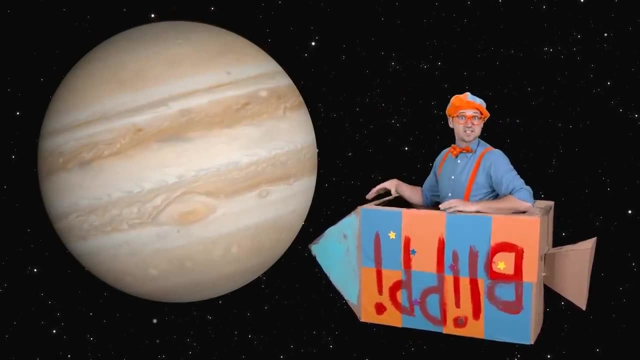 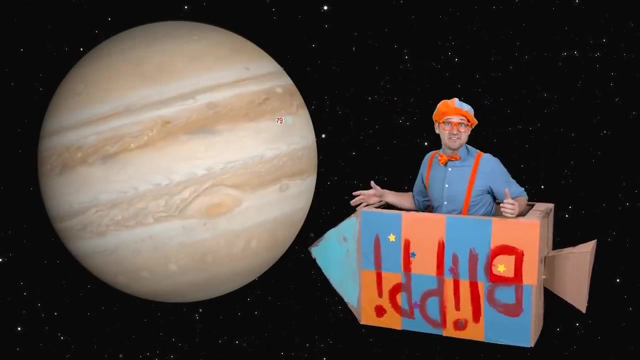 Whoa, and look at that, That's our planet, Jupiter. It's the biggest planet in our solar system And you see that big red dot. That is a storm. Whoa, That's a big storm, And Jupiter actually has 79 moons. 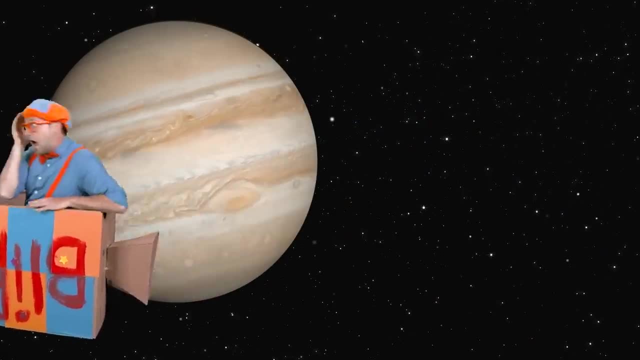 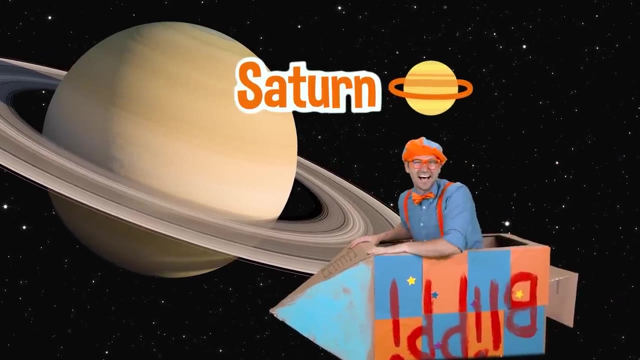 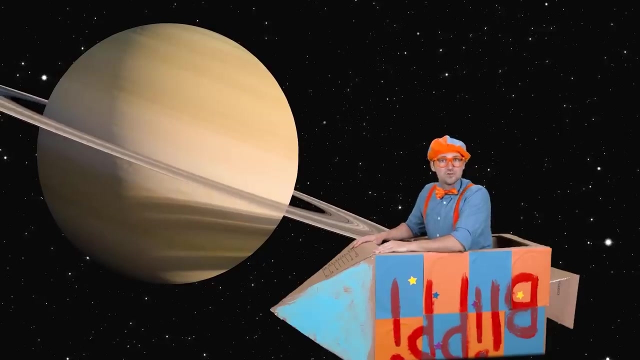 That's crazy. Whoa, Haha, Woohoo. See you later. Jupiter, Hello Saturn, Haha, Check it out. This is our planet, Saturn. Whoa, What are those? Those are Saturn's rings, Wow. 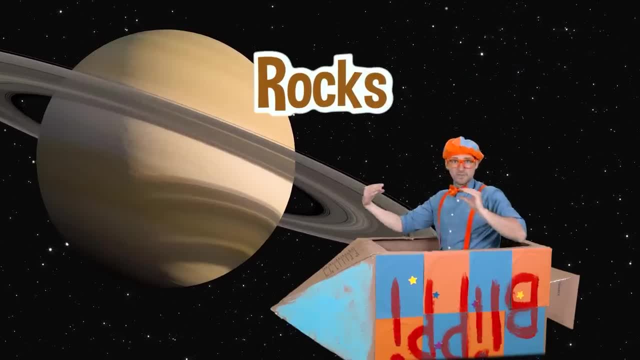 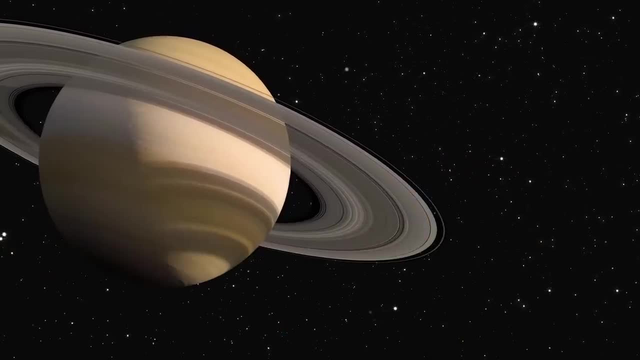 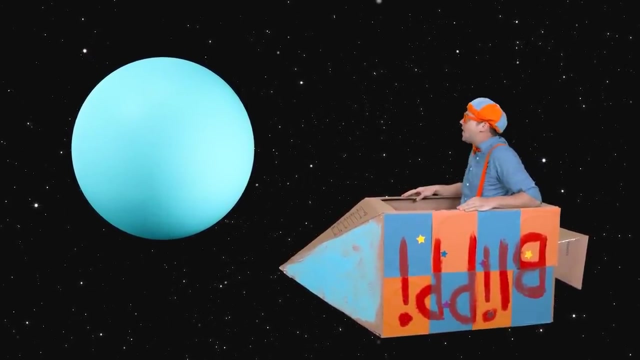 There's so much dust, ice and rocks that form those to make up those rings. Wow, what a cool-looking planet. All right, Saturn, see you later. Bye-bye, Haha, Weehee, Haha, Whoa. 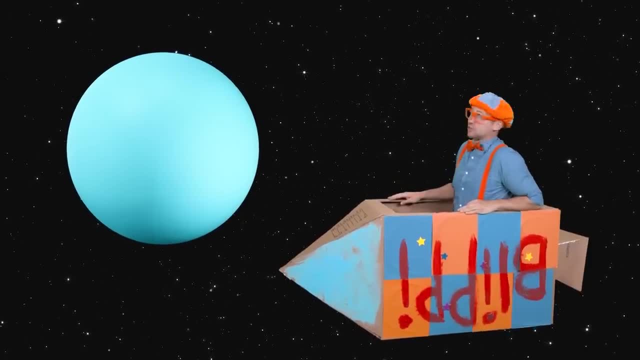 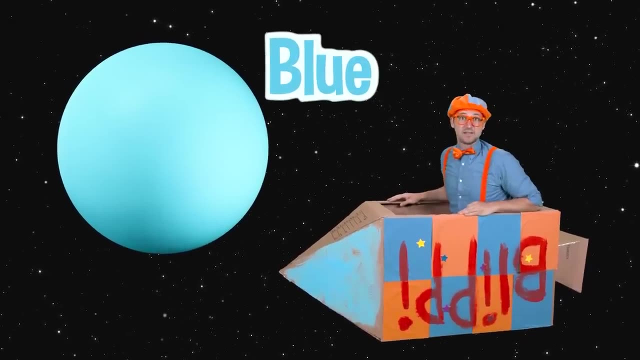 Oh look, Another planet That is Uranus. Yeah, what a cool planet. Wow, it's kind of blue-looking, huh. Yeah, that's because there's so much ice on it. It's known as the Big Ice Planet. 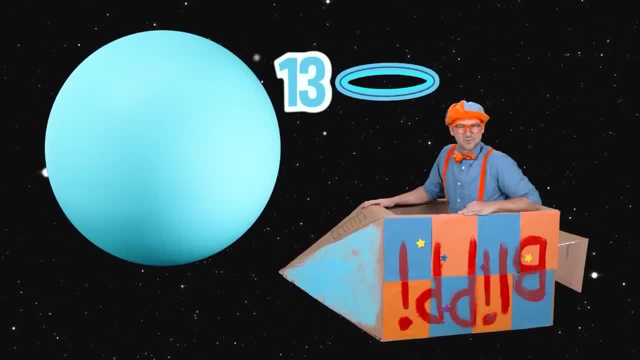 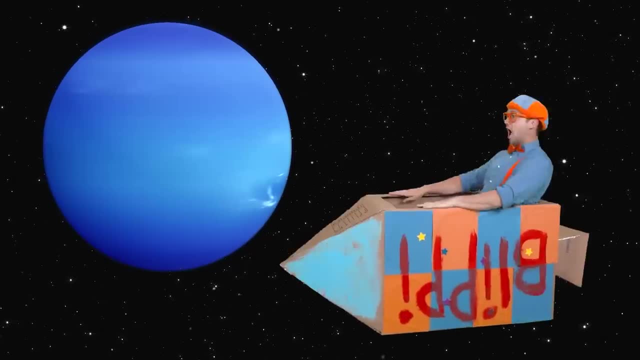 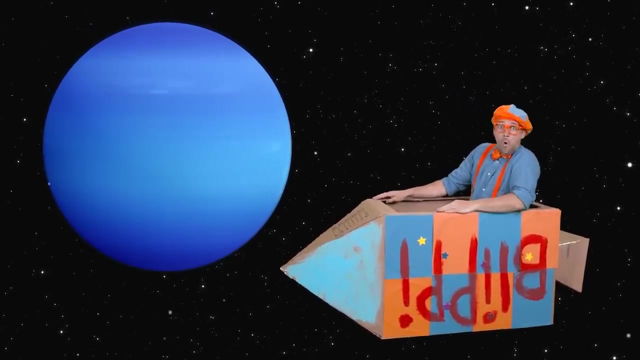 Whoa, It has 13 rings and 27 moons. All right, See you later. Uranus, Bye-bye, Oh, Whoa. Yeah, This has been so much fun. Whoa, Look at that planet. That planet is the planet Neptune. 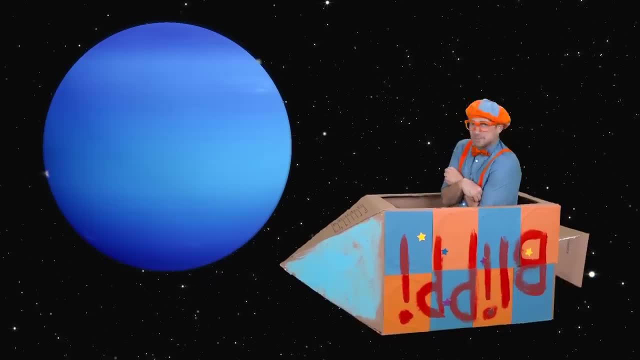 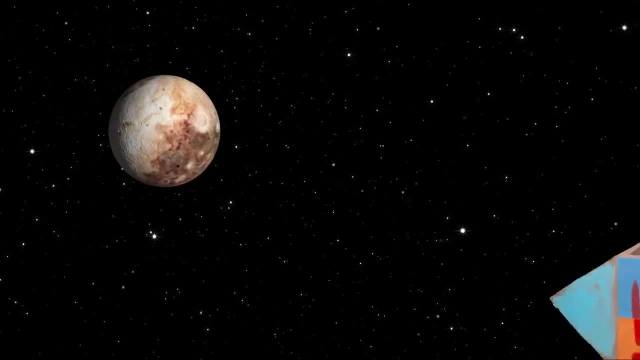 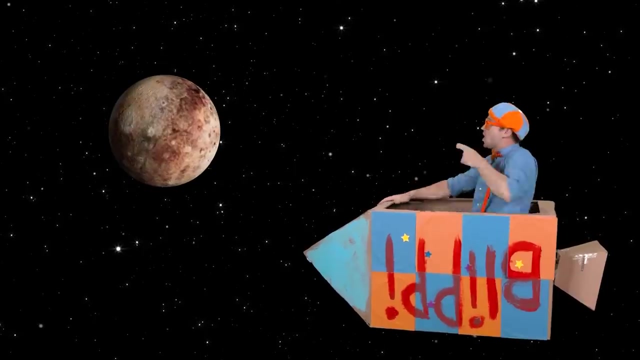 It's so dark, cold and windy I can't see on that planet. Oh, Let's get out of here. Whoa, Whoa, Woohoo. The last planet on our solar system. Look at it, It's really small. 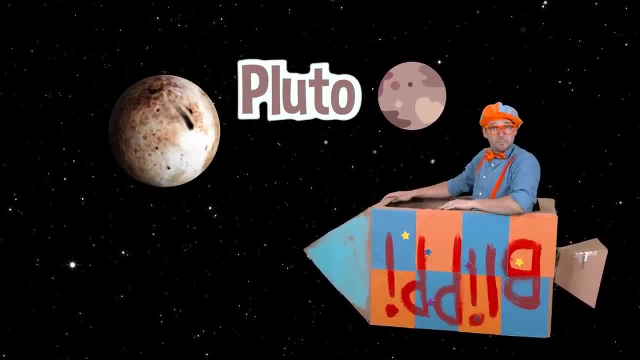 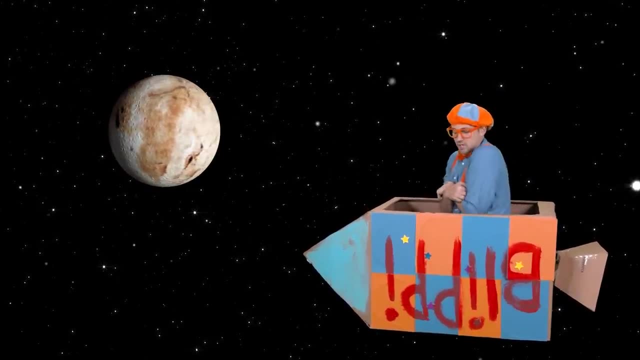 That is Pluto. It's so small, it's a dwarf planet, Wow, and it's really cold. I love Pluto, Haha, Whoa, It's really chilly out here, though Let's turn around and count all of the planets. 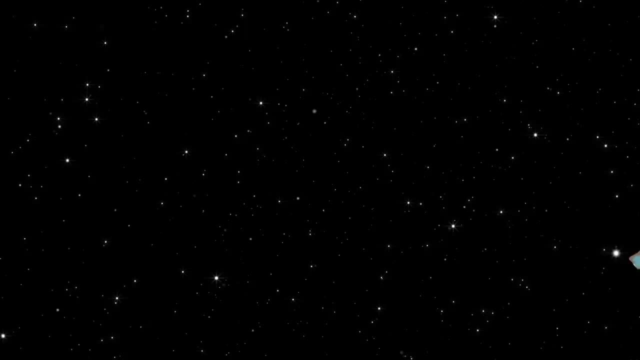 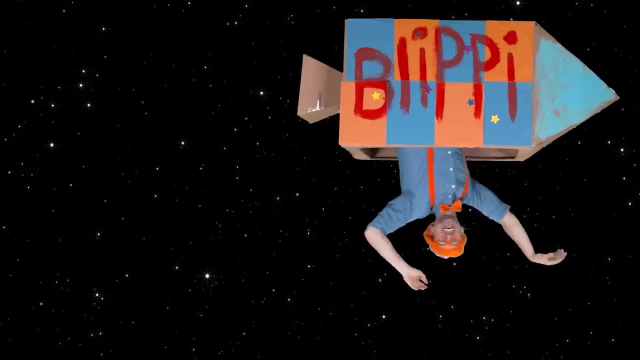 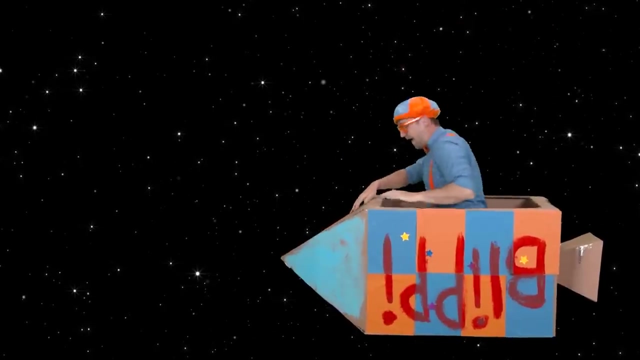 Shall we? Woohoo, Woohoo, Yay, Whoa, I'm upside down, But now look at my name. Woohoo, Haha, Whoa, Whoa. That was so much fun learning about all of the planets in our solar system together. 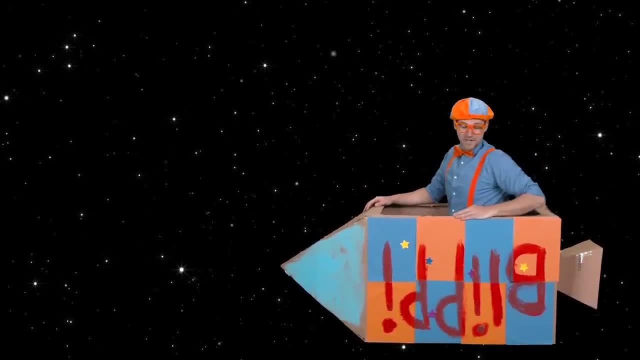 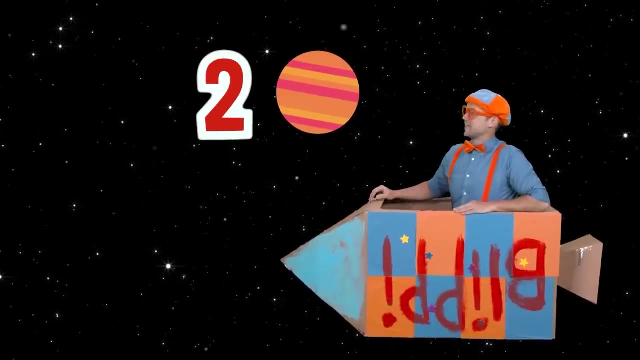 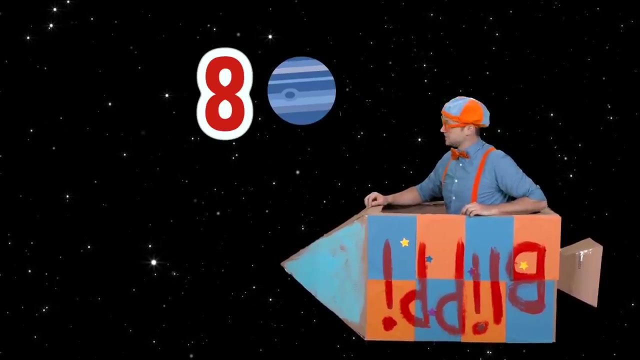 Hey, I think we should count all of them. Okay, the Sun isn't a planet, so let's count the planets One, two, three, four, five, six, seven, eight, nine. Oh Wait, a second. 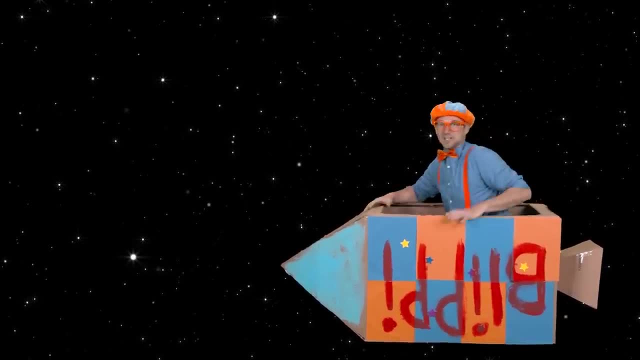 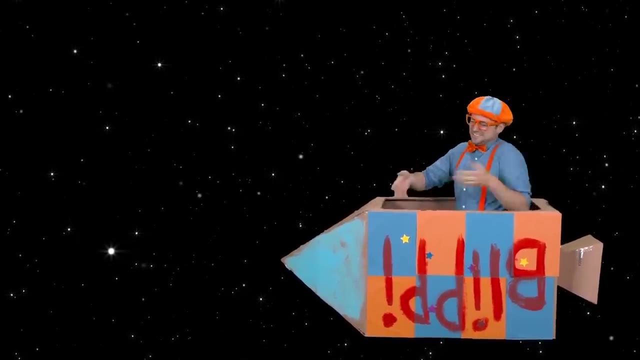 Eight, Nine, Ah, Who knows. Some people say Pluto's not a planet, but I don't know, It's all up in the air right now, Or outer space, Haha. So silly Eight or nine, We'll keep it at that. 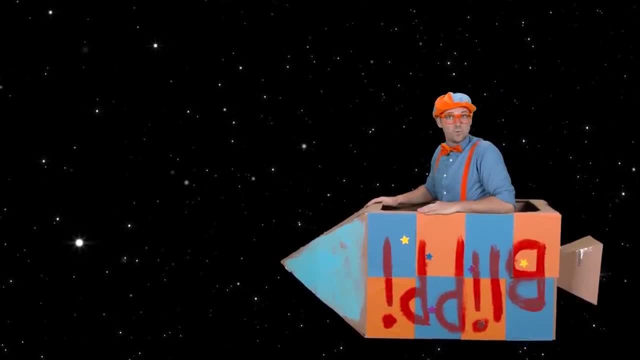 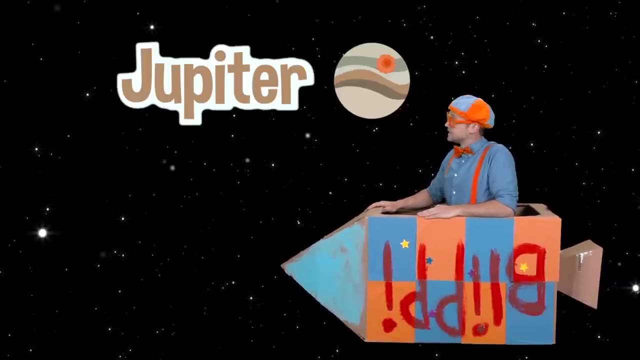 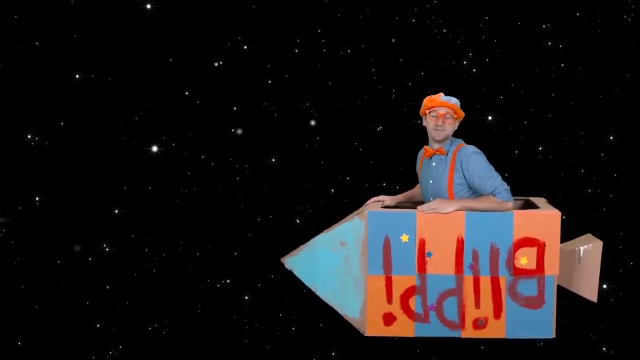 Okay, now let's name the planets Ready: Mercury, Venus, Earth, Mars, Jupiter, Saturn, Uranus, Neptune, Pluto. Wow, Good job, Alright. Well, I should probably get going now. Maybe we'll go and explore another planet. 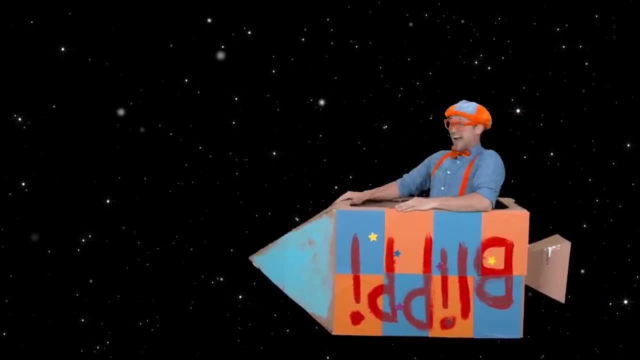 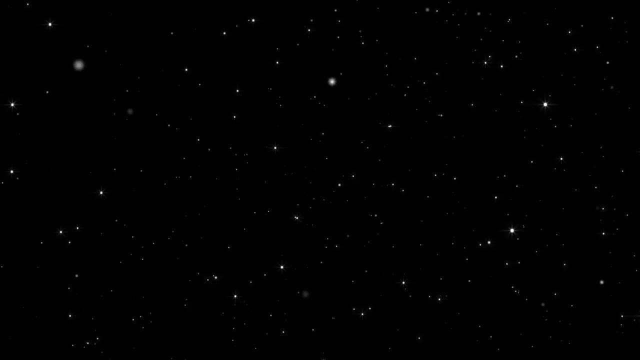 Maybe we'll go and explore another solar system someday. Alright, See you later. Bye-bye, Whoa, Woo-hoo-hoo, Yeah, Woo-hoo-hoo, Hahaha, Blippi, Come on everyone, Let's make learning fun. 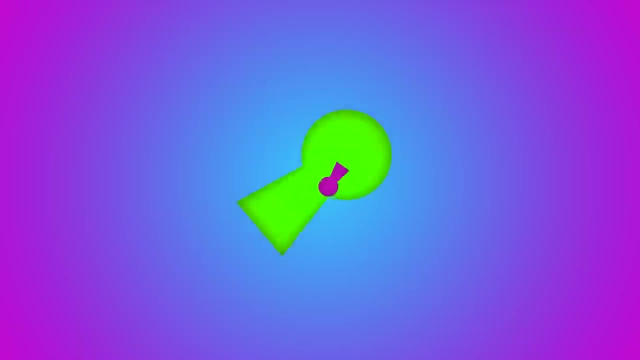 Blippi, Blippi. So much to learn about. It'll make you want to shout Blippi.